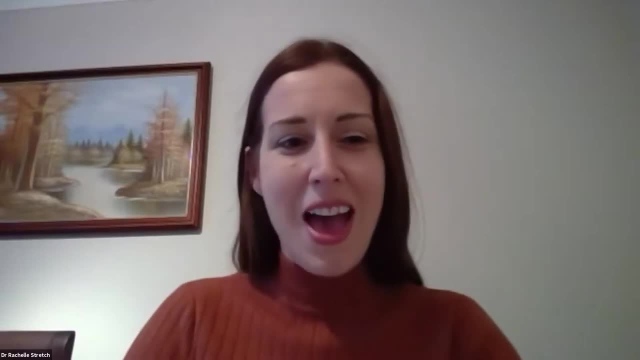 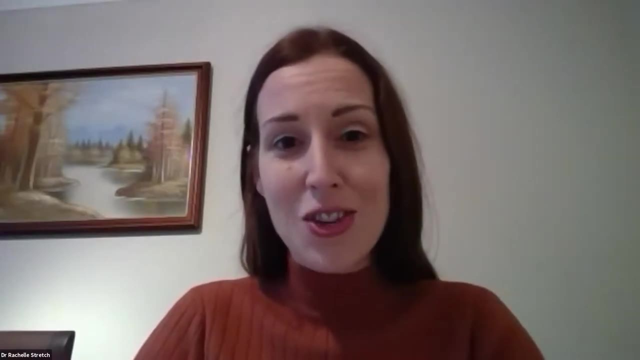 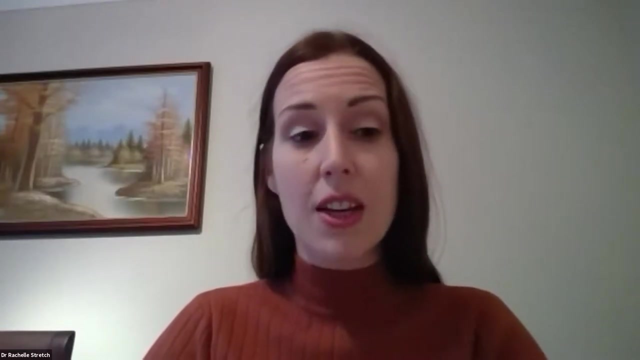 And I'm delighted that we have an event with Emma Karst, who is a Research Fellow in Geography, Geology and Geophysics at Trinity Hall and joined us last year during lockdown, But Emma didn't. She did a PhD in Geosciences from Princeton and studies marine biogeochemical cycles and ecology across the Earth's history, So I'm delighted to hand over to Emma and hear more about paleoclimate and ocean nutrients and what we can learn from the Earth's geological record. Thank you, Emma. 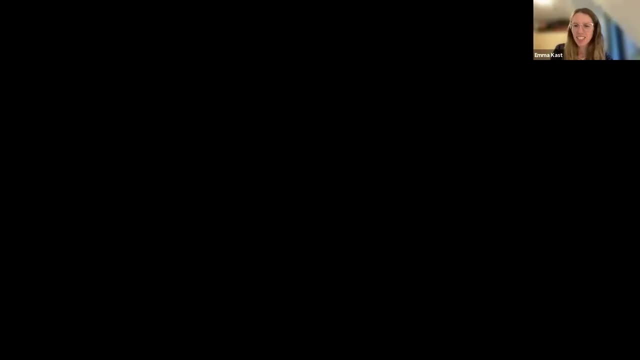 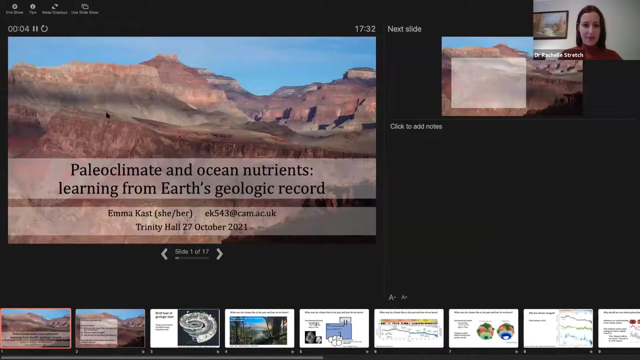 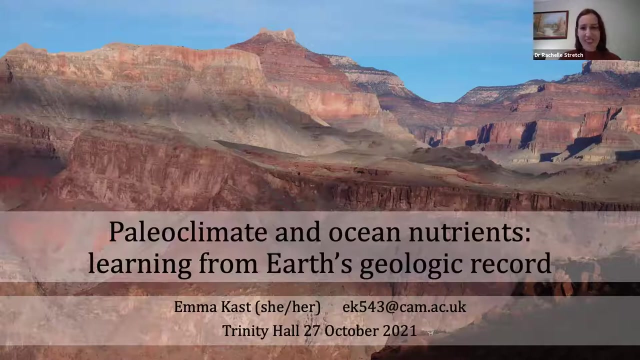 Great, Let me just share my screen. Perfect Other way. Oh yeah, Like this. Perfect, Okay, Great, Yeah, it's such a pleasure to be here and to be talking with you all. So, um, yeah, I'm going to be talking a little bit about paleoclimate in general and also a little bit about ocean nutrients. 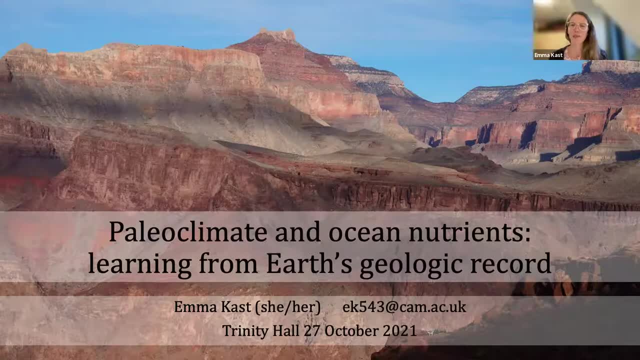 And all of this is things that we learn from the Earth's geologic record. So I'm- I'm actually from Arizona and this is a picture of the Grand Canyon, and I thought I'd start with this just because it really nicely shows these layers of sediment that built up over time. 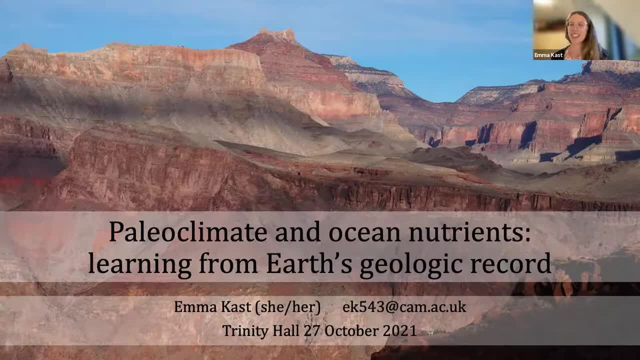 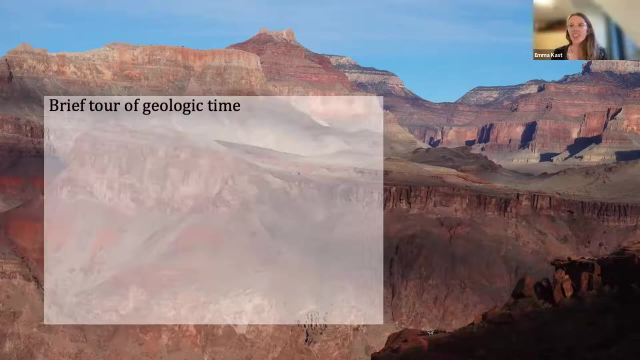 And there's over a billion years of history recorded that you can see in the Grand Canyon. So I thought that was a nice start to our our evening. Okay, great. So, um, first I just wanted to give you a little bit of a just like outlines, you know what's headed your way. 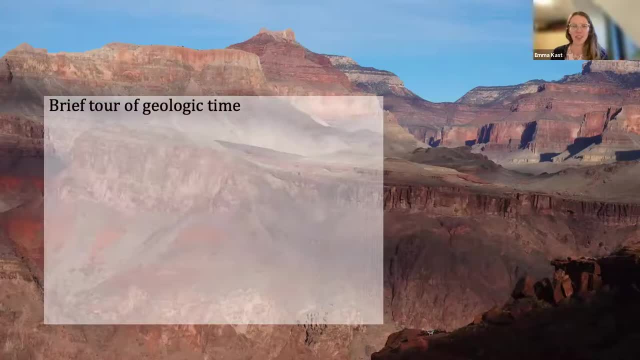 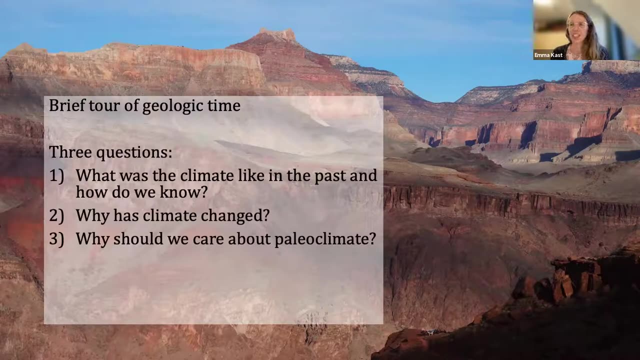 First a brief tour of geologic time, just get us all oriented on the same page, And then I really want to talk through kind of three questions. So first, what was the climate like in the past and how do we know? Second, why has the climate changed? 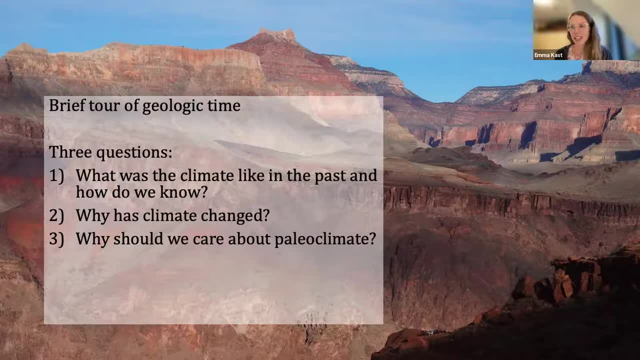 And then third, why should we care about climate in the past or paleoclimate? And then last, hopefully have a bit of time To talk about some of my own research into ocean oxygen and nutrients likely in the past. So we'll kind of wrap it up with a little kind of research example. 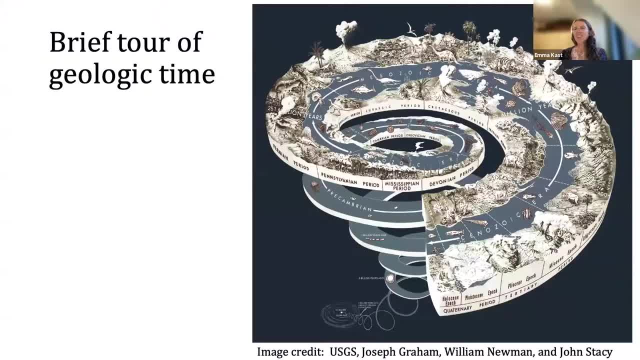 Okay, um, yeah, so a brief tour of geologic time. This is a really great figure. that kind of gives you a sense for earth history. So starting, hopefully you can see my mouse. So starting the bottom left, here Is the formation of the earth, which happened around four and a half billion years ago. 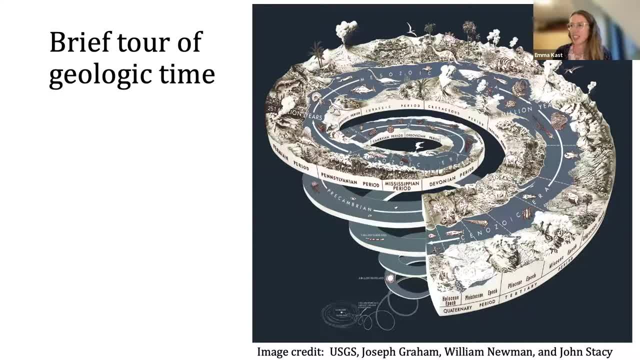 And then these spirals are basically time moving towards the present. So, on this figure, the present is this part nearest to us And I guess I just want to give you an appreciation for the amount of time that's exists in earth's history and some kind of key events. so 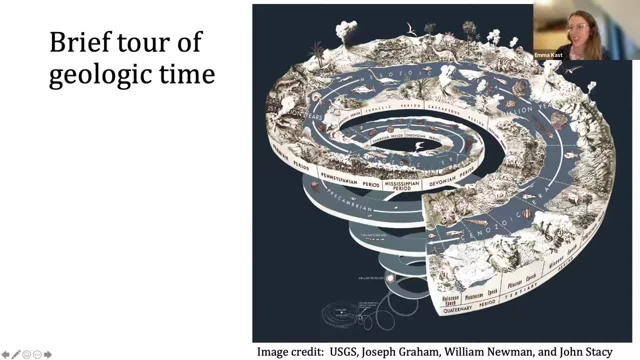 around three and a half billion years ago. So the first signs on the way down here and these little spirals are first signs of of life on earth Around 2 billion years ago. we get photosynthesis and the rise of oxygen, And we can also get some more. 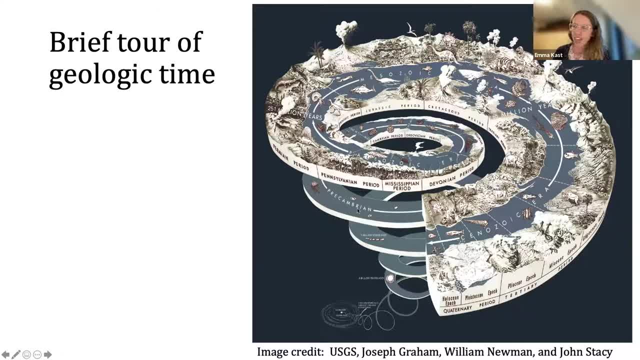 More recent events, so billion years ago, I get the first animals And as we move up the spiral You can see Kind of The Diversification of life. and today I'm actually going to be focusing on a relatively short amount of time in the scheme of 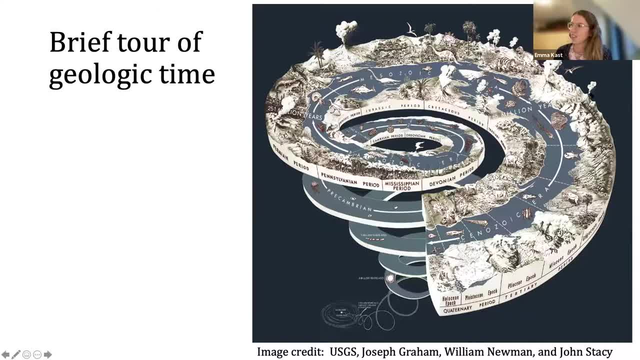 geologic history, which is basically- if you can see my mouse from this line to the present, on the last 65 million years. It's called the Cenozoic, or sometimes referred to the age of the mammals, So basically the time period from when the dinosaurs went extinct until modern day. 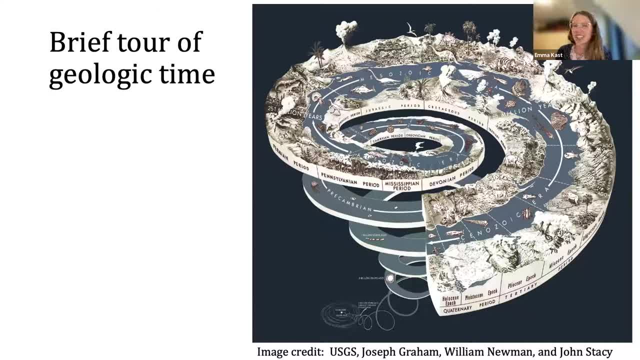 And if we want to put humans on this kind of geological time, we're all basically right at this last sliver of this diagram, Okay, so yeah, like I said, today we'll focus on last 65 million years and the climate over the Cenozoic on a pretty long time scale, Okay, 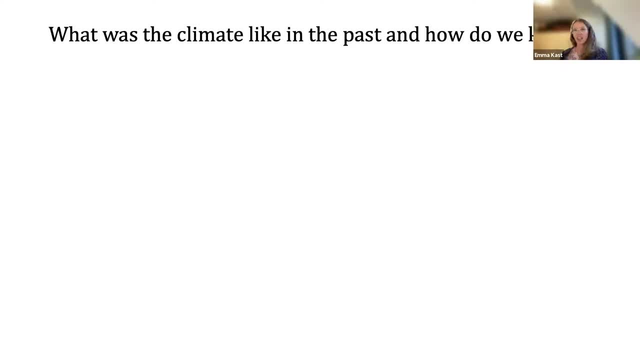 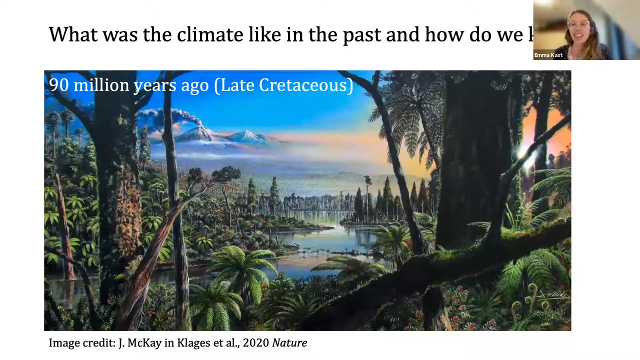 Okay, so the first question: what was the climate like in the past And how do we know? And the first example that I want to show you is actually this: it's an artistic reconstruction of an environment somewhere on earth 90 million years ago. And so, while I'm talking through this figure, 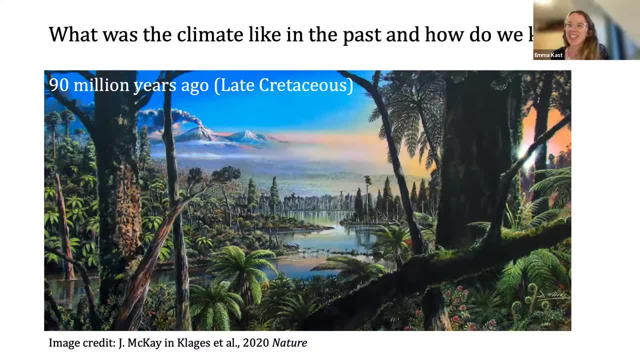 I, in your head, try to guess which continent this reconstruction is from. So the way that this was made is basically: some researchers found a bunch of fossils of different plants, So things like terns and woody trees- and they use these to infer that this location must have been this kind. 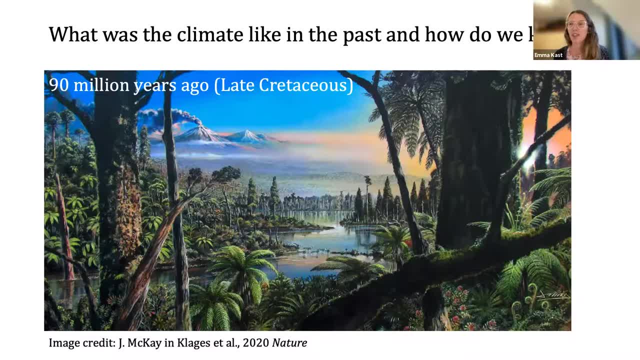 of temperate rainforest type environment, And so we kind of have a sense for the climate of this place based on what plants and animals existed at that time. Now the surprising thing is that this is actually a reconstruction of West Antarctica 90 million years ago. So it's actually a reconstruction of West Antarctica 90 million years ago. 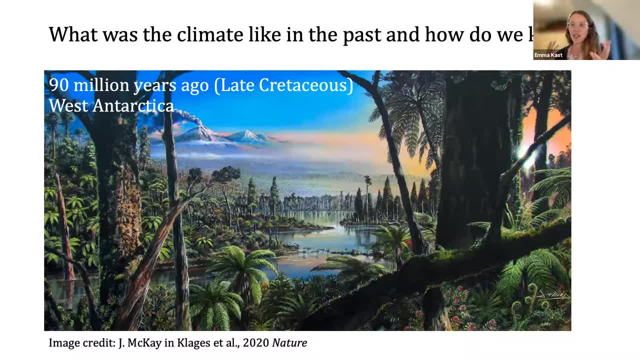 ago. So if you were to go there today, instead of this kind of lush plant life, you'd find basically more than a kilometer thick ice sheet on top of the land. So clearly like dramatic changes in climate over these kind of time scales. 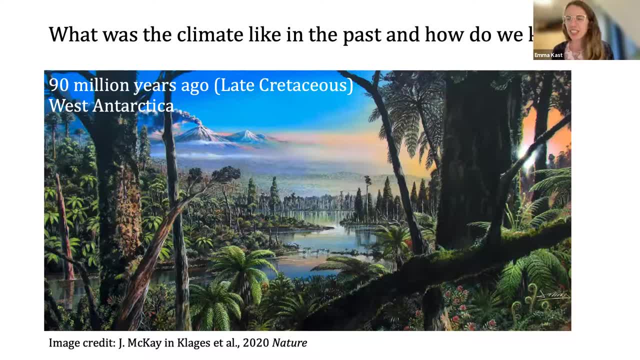 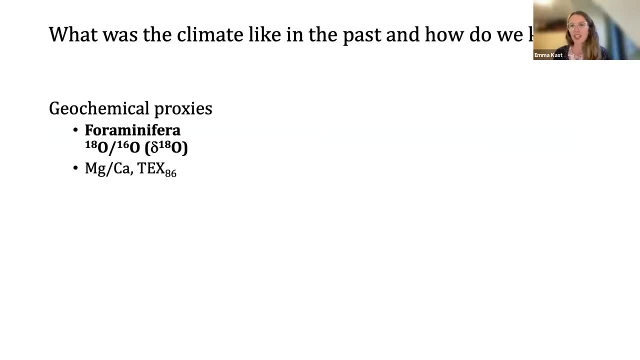 Okay, so this is kind of one way we can learn about climate in the past, is, you know, looking at what plants were around and trying to infer what types of environments they would have been able to live in. However, we have a lot of other tools as well. Really, the big ones are these: 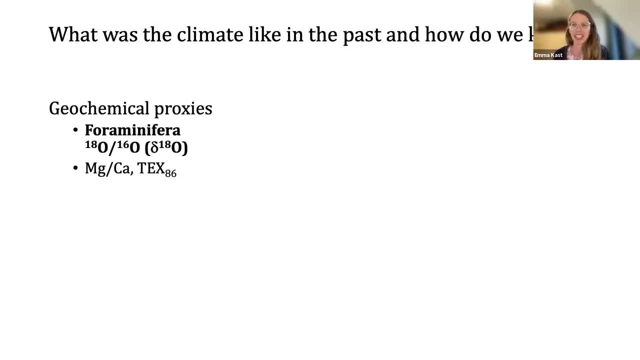 things that we call geochemical proxies. So a proxy is a way you can learn about the climate, kind of like by measuring something else. So some of the big ones in terms of reconstructing temperatures. the first one is the oxygen isotope composition of something called foraminifera, And I'm going to 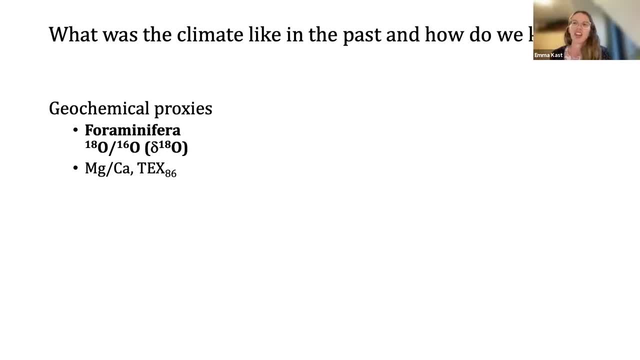 talk a lot more about that in a few seconds. And then there's other varieties of proxies as well, So you can look at magnesium calcium ratios in different kind of fossil materials. There's different biomarkers that you can look at and try to reconstruct temperature that way too. So there's 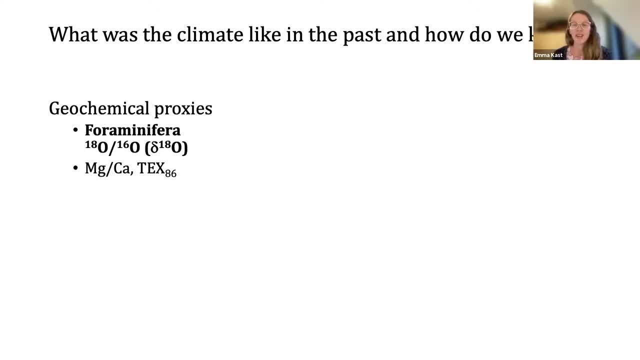 a whole kind of suite of proxies that we use to try to reconstruct temperature. So one of the most fundamental ones, and that's been used really widely in the field of paleoclimate, is this: foraminifera- oxygen isotope proxy. So what is is So? first, foraminifera: there are these tiny animals, So they're around. 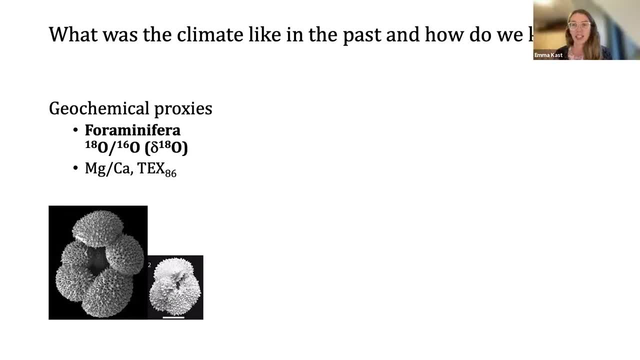 them with your eye, but they look like a tiny, like speck of sand, basically, and they're really cool because they form this carbonate shell and those shells can get preserved in marine sediments and then we can go out into the ocean and basically bring up these ancient shells and measure their 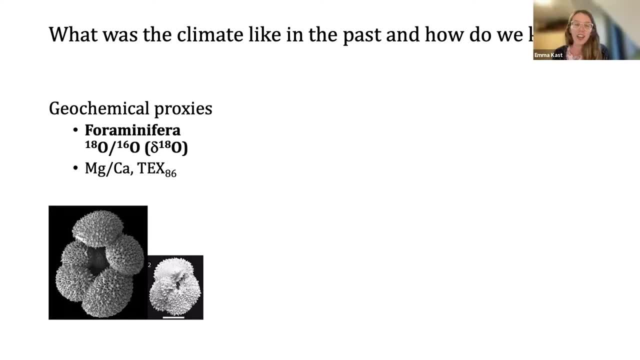 chemistry to try to figure out stuff about the climate in that way. okay, so that's the for maneuver part. so what about the oxygen isotopes? so the oxygen isotopes work like this: this is the lovely ocean, as you can clearly see by my square blue box, and the water in the ocean can. 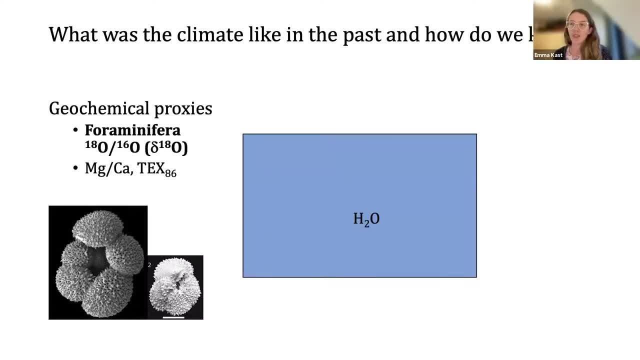 have one of two isotopes on the oxygen atom can have oxygen 18 or oxygen 16. and when there's ice on the planet like this, they tend to um. the lighter isotope, the 16-0, tends to preferentially end up in the ice and versus the ocean. so this creates this kind of relationship between the. 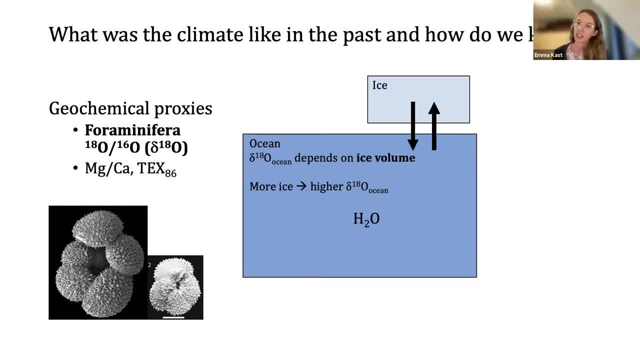 amount of ice and the oxygen isotopic composition of the water in the ocean. so basically, more ice. it means you have a higher um 18-0 to 16-0 ratio or a higher delta 18. which is just the type of notation that we tend to use. so that's one component um, and then there's 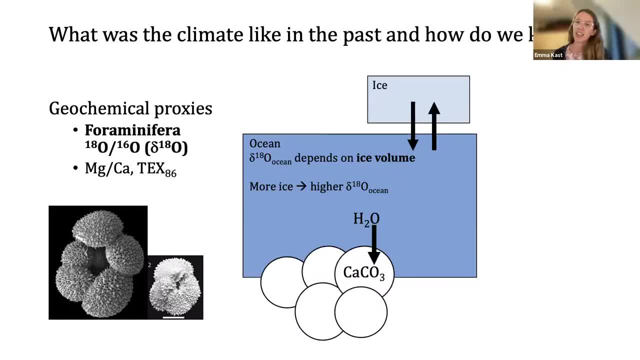 another component, which is how that oxygen actually ends up in the carbonate shell of the foraminifera. so i'm representing that by this arrow between the oxygen in the water and in the carbonate. this is the molecular formula for carbonate and those two things are in equilibrium. 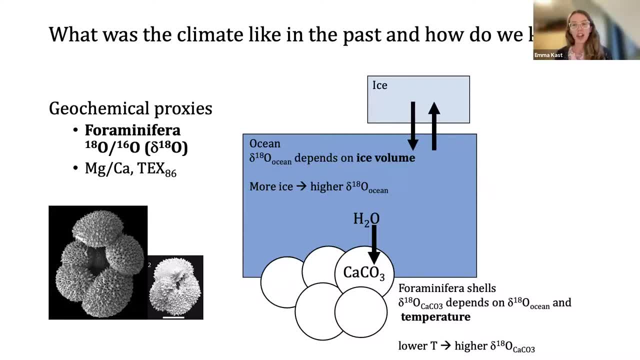 with each other and there's a temperature dependence to the way that the isotopes into the carbonate and just uh, simply, if it's a lower temperature in the water, then the carbonate is going to have a higher delta 18.. so this is kind of the mechanisms at work behind these. 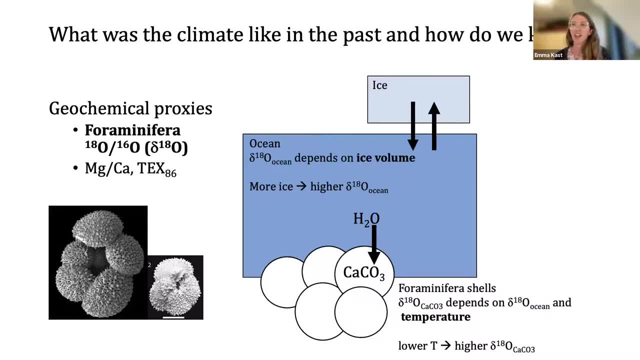 geochemical proxies. i think it's really nice to kind of get an understanding of how these work, because the next thing i'm about to show you is a record, over the past 65 million years, of how this foraminifera oxygen isotope value has changed. 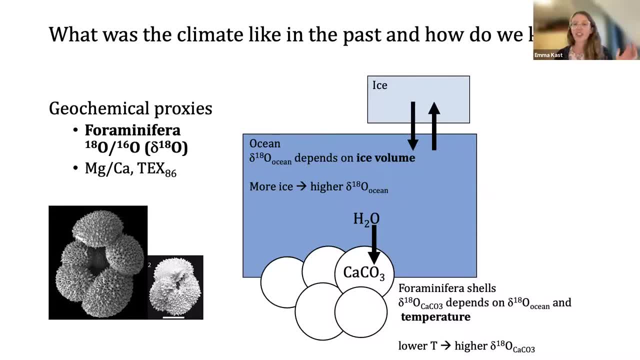 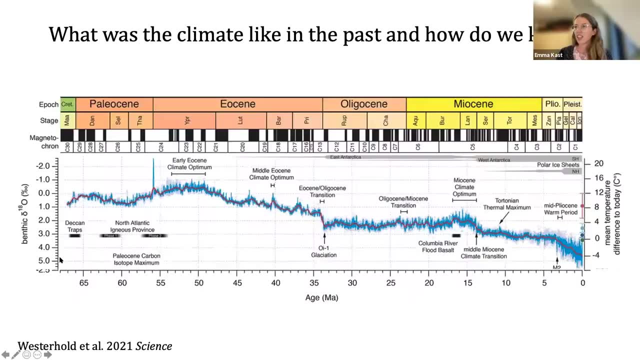 over time and we're going to see what was going on with temperature um across the center. okay, all right, we will talk through this figure together. so, to orient ourselves on, the x-axis is age, so the oldest part is over here, which is 65 million years ago. 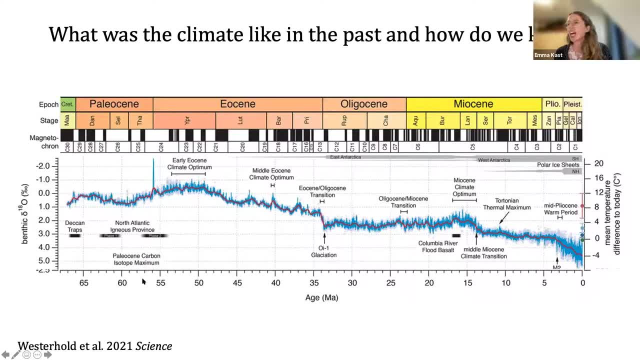 so this is like the dinosaurs went extinct here, and then all the way over to the right side is modern day, so zero million years ago. and then on the y-axis is this: i think on this figure it's called benthic um delta 18, but that's the foraminifera delta 18, so the 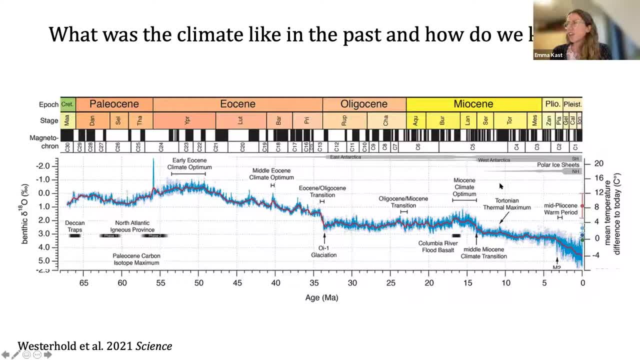 thing we just talked about, and on the right side there's actually a temperature axis. so the authors that created this figure basically transferred or calculated the temperature from this oxygen isotope. the stuff in the colors at the top is just the names for the different eras and 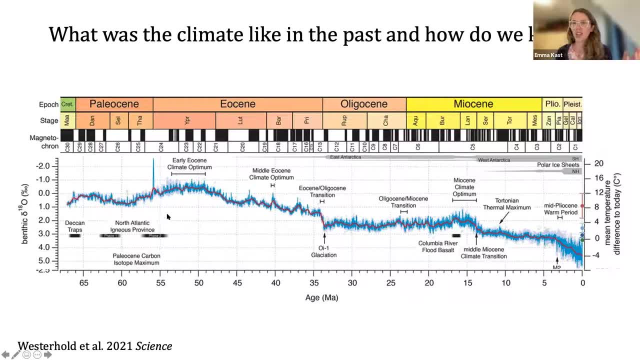 we don't really need to worry about that too much. okay, so i just want to describe some broad trends, um about. you know what was going on in the cenozoic in this last 65 million years? so early on, temperatures were relatively high, so around, let's say, eight degrees celsius. 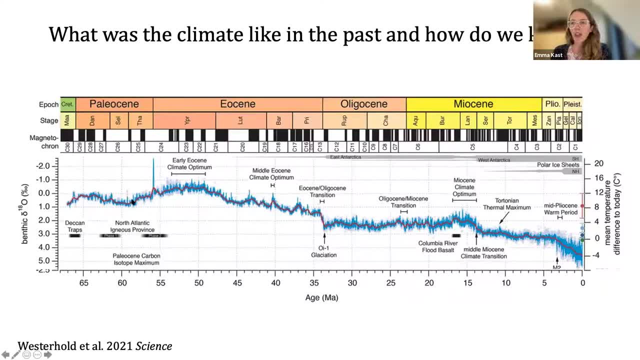 higher on average than modern day. at the beginning there was a bit of warming up until this thing called the early eocene climate optimum, which are kind of our warmest stable temperatures in the cenozoic. there's also this really dramatic event, um really like abrupt warming event that happened um in the early cenozoic, called the paleocene eocene. 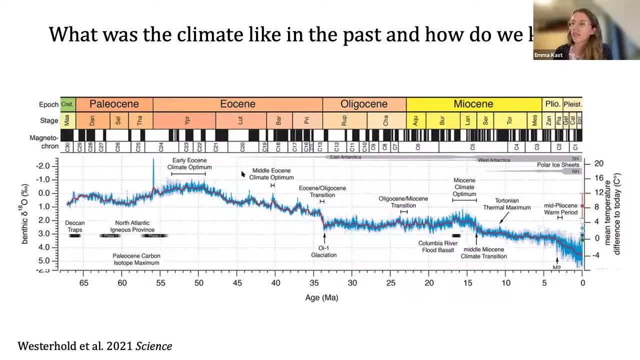 thermal maximum, the phm- um, and then the- the majority of the trend of uh climate over this time period is really a long period of time and that's why it's called the early eocene climate optimum- um, and then the the majority of the trend of uh climate over this time period is really a long. 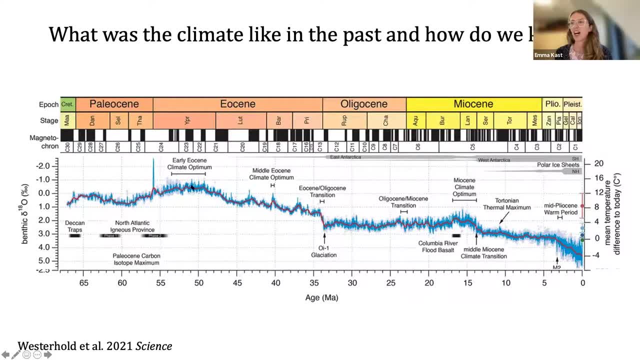 term cooling. so from this early eocene climate, optimum kind of had this steady cooling with you know some stepwise things as well, um, steady cooling all the way down to present day. okay, some other things to point out that are on this graph are these gray bars and these are our best. 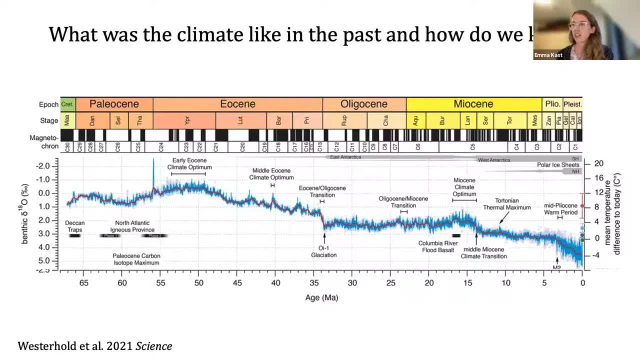 understanding of when we started to get ice sheets on earth. so antarctica started to be glaciated around this time, in kind of the middle of cenozoic, so around 35 million years ago, and then much more recently the northern hemisphere ice sheets really started to pop up around two and a half million years ago, and this is when we get the. 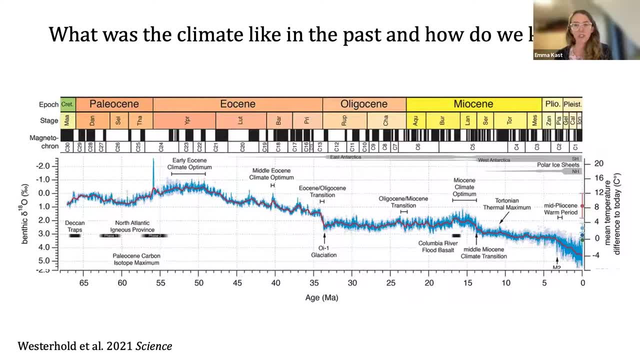 start of the glacial interglacial cycles, um, that i'm sure most of you have heard about in some context and so this like really high variability signal here. those are glacial interglacial cycles and again, this is a big picture for global climate studies and i think some of you know. 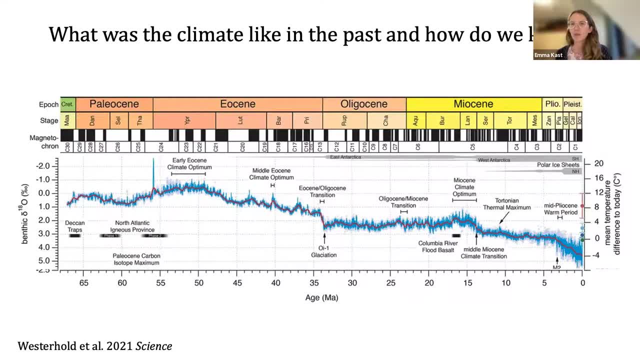 these are a record of what happened over the last few decades, and so i'm going to put together some of these charts and then give you the next slide so i can share you the feeling of your recording when you get to the end of the slide, and to know what's going on with global climate. yeah so, 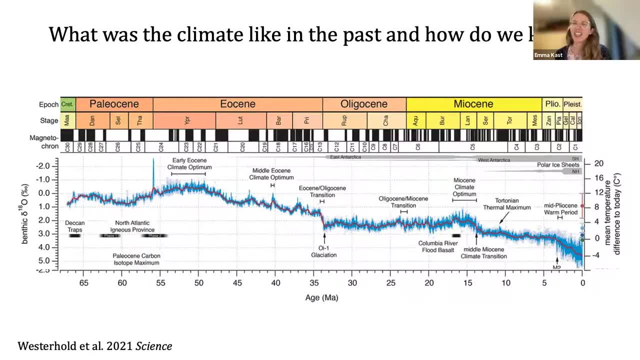 for instance, i was talking about the cold winter, days of the winter, because i was thinking, like you know, it's gonna be a very hot spring and it's gonna be a very cold year. it's gonna be a very warm year in the winter days. and i want to talk about some of the things that are happening in the 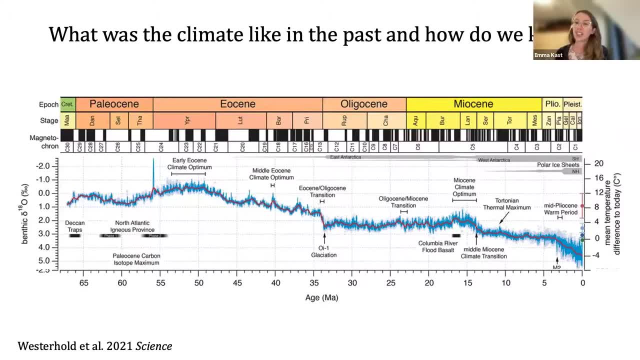 We want to know local things. so how is the temperature distributions different at different times? There's also other aspects to climate, so things like precipitation or humidity that really aren't captured at all in a proxy like this. So sometimes we need other tools and I can't obviously go into like all the different ways that we can learn about. 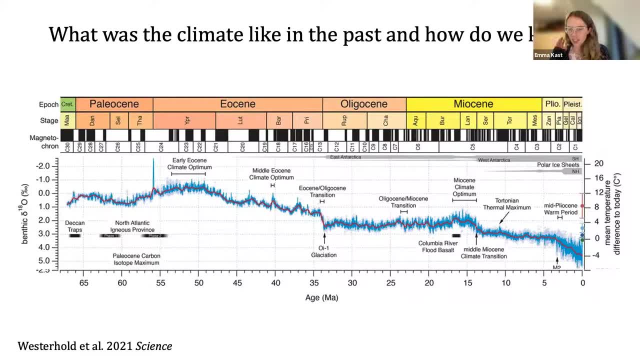 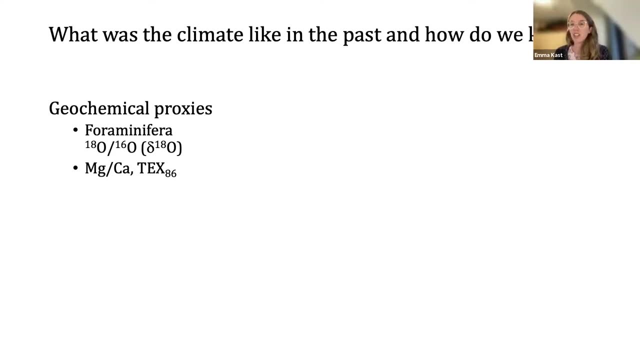 climate. but just to say that this is one of our- you know- key understandings of Cenozoic climate, but it is also kind of a small piece of the overall puzzle, Okay. so yeah, we touched on geochemical proxies, and I wanted to mention one other thing that we're really starting to do in a more rigorous way with paleoclimate. 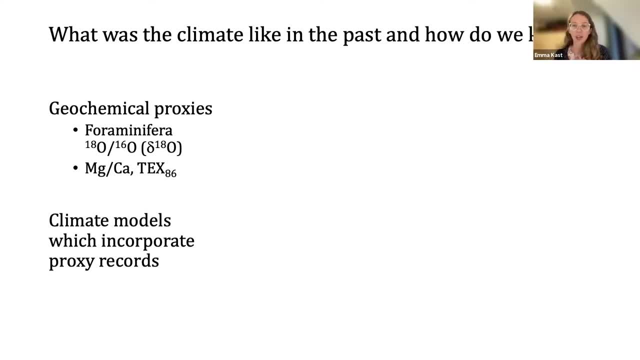 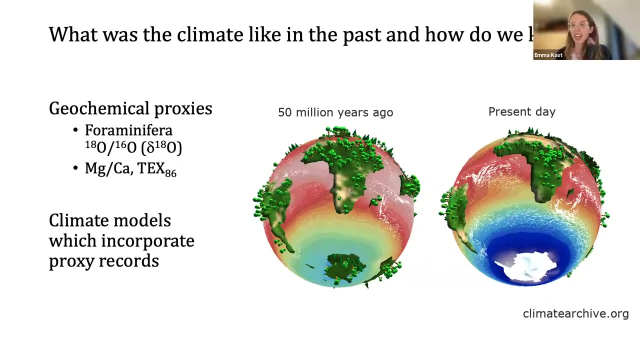 which is to use climate models that can actually incorporate these proxy records To kind of start getting a more holistic sense of what climate was like all over the globe. So I think you've actually perhaps seen this picture, because it's the image I reused for the kind of advertisement for this talk. 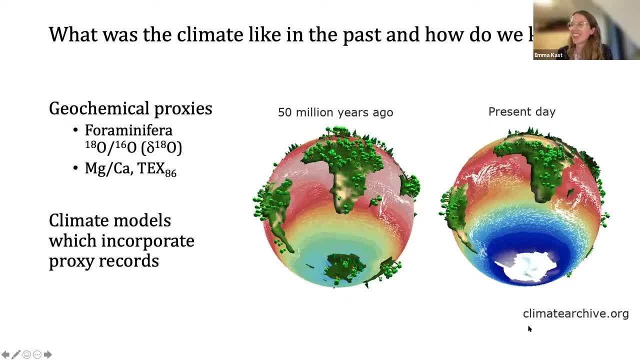 So it's a really cool website. I would encourage you to check it out. It's called climatearchiveorg and you can basically play around with what models are saying about paleoclimate over the past, So I just kind of grabbed a couple screenshots of 50 million years ago. 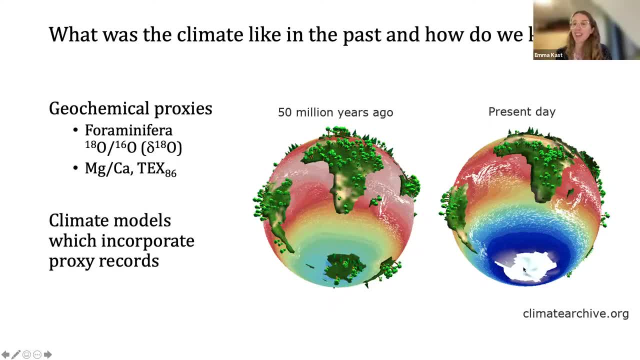 and the present day. You know, one big feature you can pick out is that 50 million years ago, no Antarctic ice sheet, and even you know vegetation differences and all that kind of stuff are incorporated into these models. Okay, Okay, so to move on to the second question: why has climate changed? And when I'm saying this question? 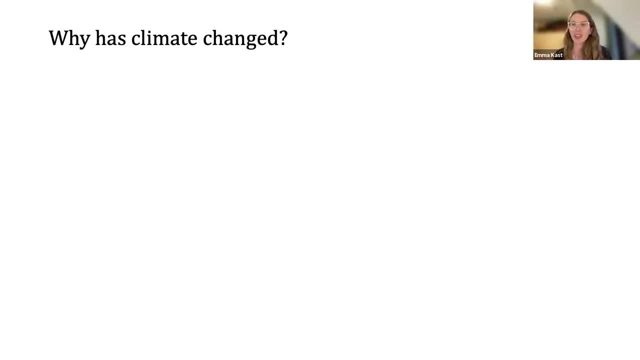 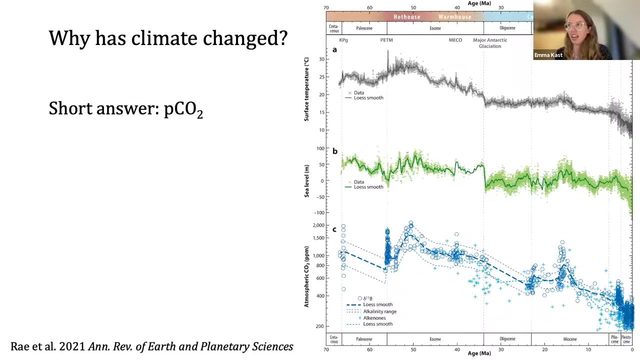 I mean, why is climate change over this? you know specific time period that we're looking at, the last 65 million years ago- And, to be honest, the very short answer to this is PCO2.. So, particularly recently, there's been some really nice efforts to reconstruct atmospheric PCO2 over the same time intervals, And so I'm going to show you a figure about that now. So again, 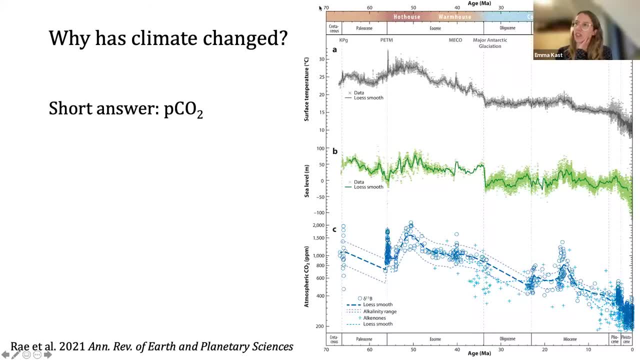 let's talk through this. So same thing with the age. So now we're starting at 70 million years ago and going up until the present. This top panel here in the gray is showing us surface temperature. So this is actually exactly the same curve that we looked at just a few slides ago. So this is a reconstruction of temperature based on oxygen isotopes and forminifera. 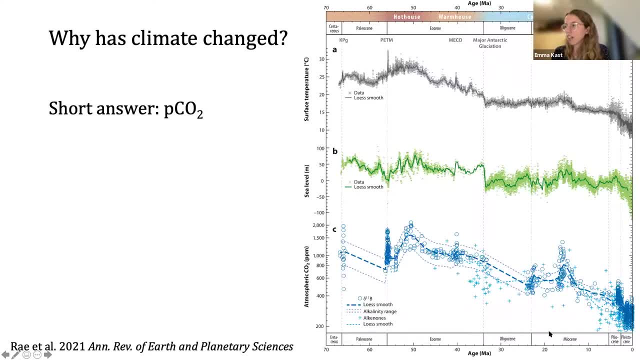 This green curve is sea level and then down here in this bottom panel is reconstructions of atmospheric CO2. over the same interval There's a few different kinds of geochemical proxies that people use to reconstruct CO2. And this is kind of our best understanding of what CO2 is doing And overall people have found is that there's a really nice relationship between temperature and CO2 and that much of the stenozoic 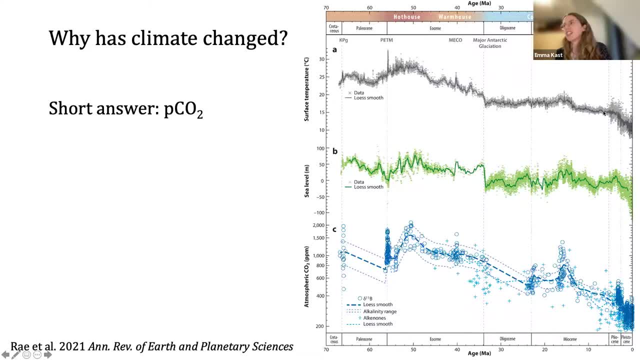 temperature changes. So you know there's warm temperatures, decline to lower temperatures Can really adequately be explained by changes in CO2 that are happening at the same time. Okay, so that's kind of the short and sweet answer to why has climate changed over the stenozoic? 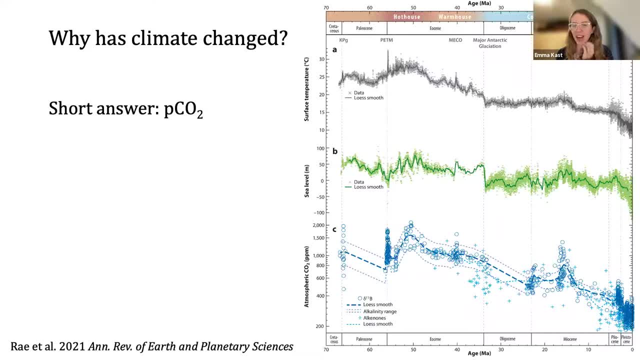 There's obviously a longer answer perhaps, and we can talk about this later if you are interested. but, of course, like, the next question to ask is: well, okay, great, CO2 has changed, but why has CO2 changed? And that's like really definitely. 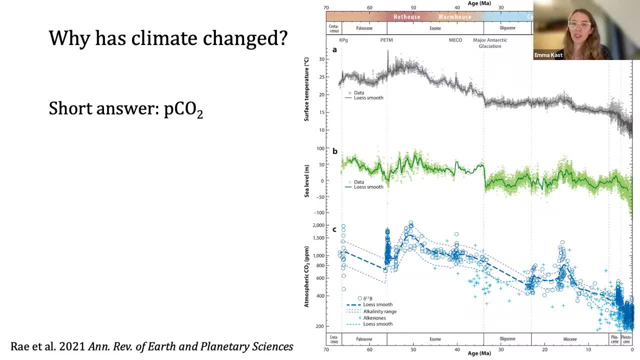 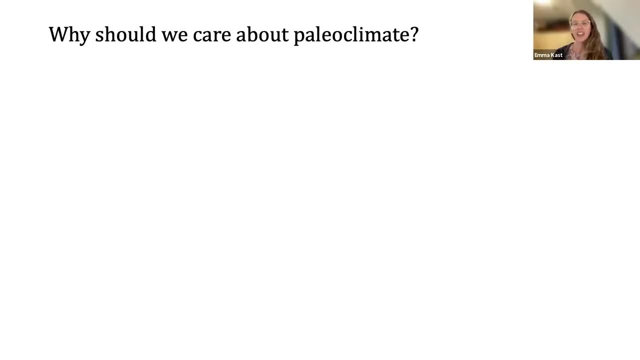 a topic of current research that people are, you know, really trying to figure out, you know, why these long term CO2 changes have happened over Earth's history. Okay, um, great. So kind of one last question in terms of: yeah, this like broad overview of paleoclimate on the stenozoic time scale. 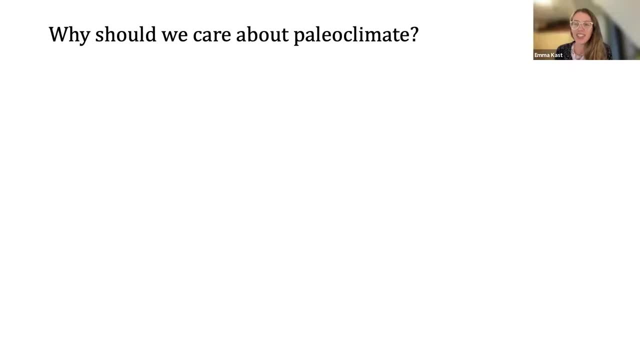 So, yeah, why? why should we care? why does it matter what the climate was like In the past? and just a couple points. So first is that by understanding the climate in the past, we actually gained some really like much deeper understanding into the climate system itself, So how it works and what the climate is sensitive to and things like that. 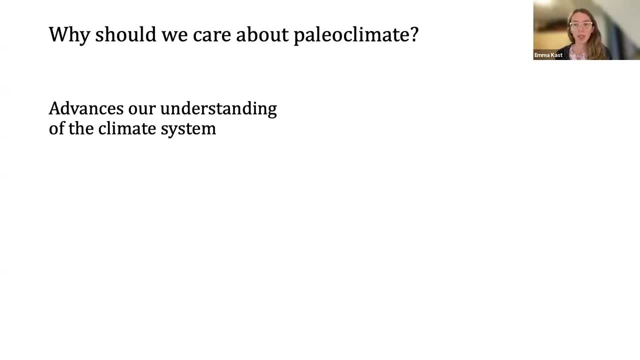 A good example is this relationship between temperature and PCO2 that we can understand better if we use the information from climate in the past. The second thing Is that these past climates can be really useful analogs for future climate scenarios. There's a really nice review paper out on this, if you're interested in this particular aspect of paleoclimate, by Tierney et al, which just came out in 2020, called Past Climates: Inform Our Future. 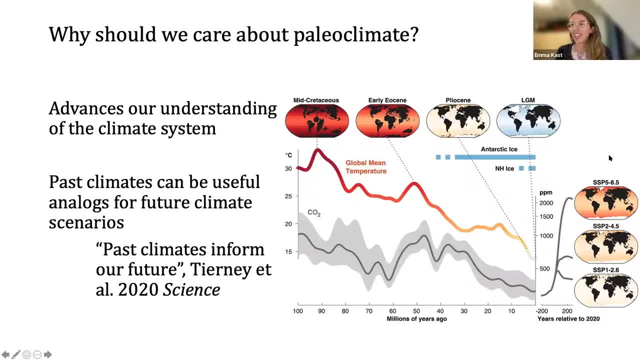 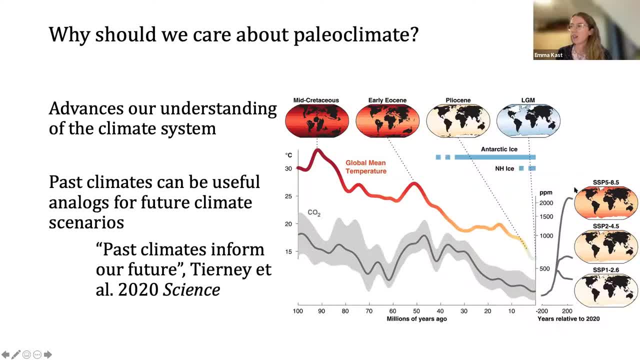 And then on this right side of the panel, what we see is a low emission scenario, a kind of mid range emissions scenario, and then a very high emissions scenario. And so one of the things we can start to do is think about, you know, as we move into the future and our modern climate is changing, how can these past times kind of inform us in terms of what future we're facing? basically, And so one of the things we can start to do is think about, you know, as we move into the future and our modern climate is changing, how can these past times kind of inform us in terms of what future we're facing? basically, 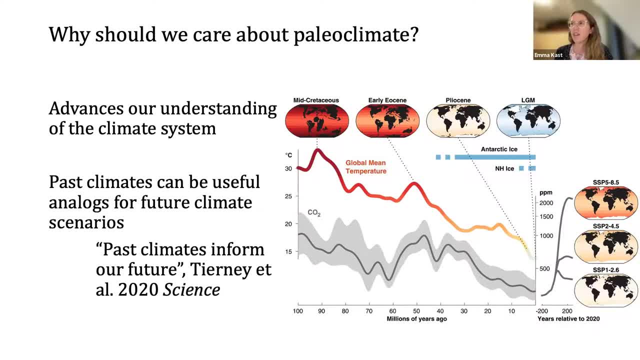 Okay, so that's um, that's what I have on the kind of, you know, paleoclimate in general type of discussion, And then I'm going to talk, hopefully briefly, about some research that I'm currently involved in. Okay, 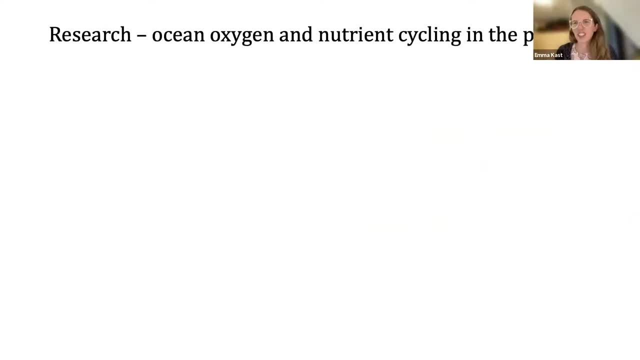 Okay, yeah. so, um, this is going to change gears a little bit, but it's really going to tie into climate. So, like, come along with me for this. Okay, so we're going to be looking at ocean oxygen and nutrient cycling in the past. 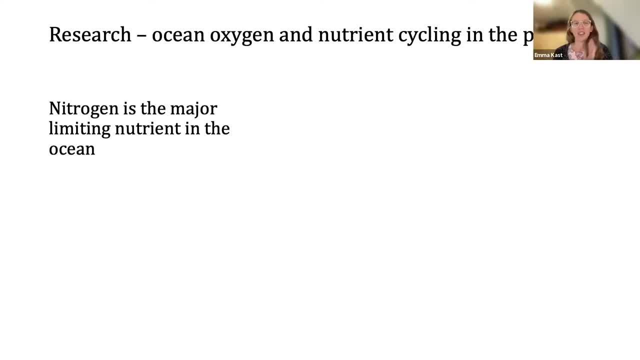 Okay, so as just some basic background, so in the ocean, nitrogen is basically the major limiting nutrient. So what that means is that if there was more nitrogen, you could have more biological productivity. So nitrogen is what's limiting biological productivity in the ocean. 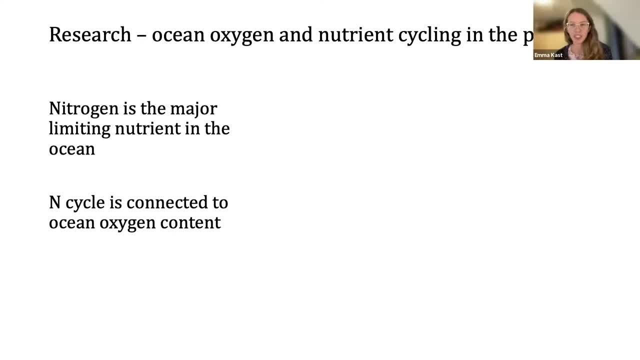 The second thing is that the nitrogen cycle is really intricately related to how much oxygen is in the ocean, and ocean oxygen has lots of implications for basically biological viability And if you have really low oxygen concentrations it's really bad for a lot of living organisms. 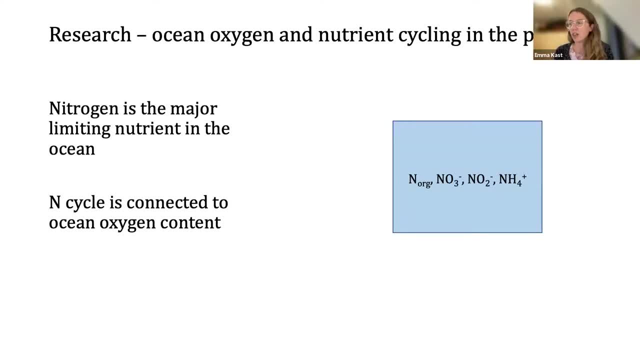 Okay. so to give a brief description of the nitrogen cycle, so that we can try to reconstruct the nitrogen cycle to the past, I'm again going to use my lovely square blue ocean to give you a sense for what the nitrogen cycle does. So in the ocean there is a variety of 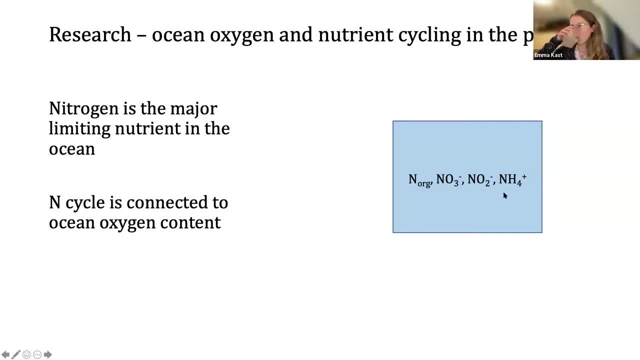 nitrogen compounds, Sorry, And these are all biologically available. And the way that nitrogen enters the ocean is through a process called nitrogen fixation, and it basically takes nitrogen that's in the atmosphere and turns it into these biologically available nitrogen forms. On the other hand, nitrogen leaves the ocean through two processes. 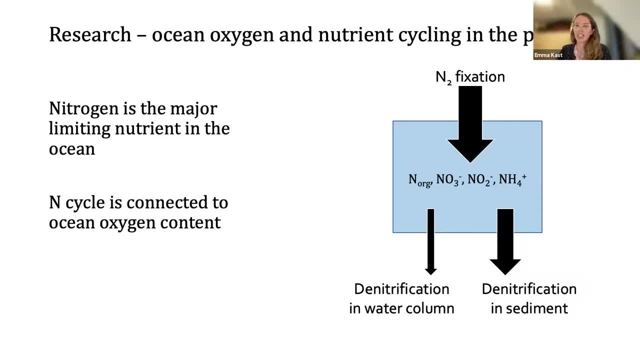 They're actually the same biochemical process, which is called denitrification. It's essentially the opposite of nitrogen fixation. it just removes the nitrogen from the system. but it can happen in two different places. so it can happen in sediments and it can happen also in the water column of the ocean, so like in the actual water of the ocean. 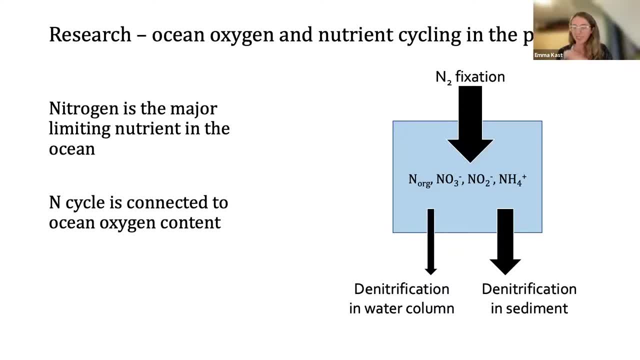 And excuse me, I'm sorry. Yeah, sorry, Okay, so the denitrification has to happen somewhere where there's really low oxygen concentrations, and in the sediments. most sediments tend to have low oxygen, which is why it can happen there, and then in the water column there are these like key regions of the ocean where the oxygen concentration goes really low and you can start to get denitrification there as well. 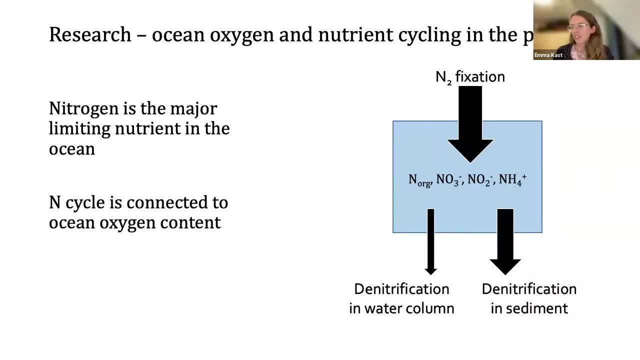 Okay, so the last kind of background to introduce here is more isotopes. So we really love isotopes, And so to reconstruct the nitrogen cycle, we're going to turn to this isotope ratio of nitrogen, so the 15 nitrogen relative to the 14 nitrogen, And, yeah, we usually call it the delta 15.. There's really only one key thing to know here, which is that denitrification that happens in the water column. 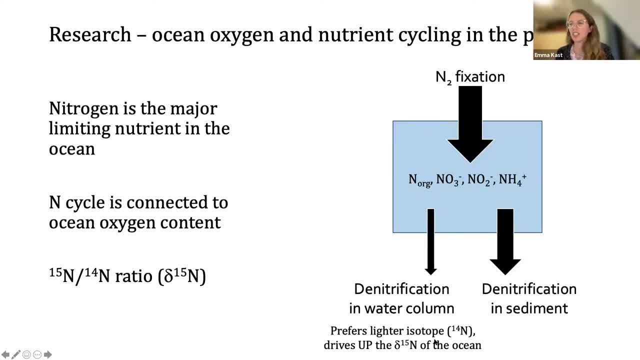 tends to prefer the lower nitrogen, So that's the lighter isotope, that 14 nitrogen, And so when you get more of this denitrification in the water column you tend to increase the delta 15 of the ocean. So basically, that remaining nitrogen, that's like leftover in the ocean. 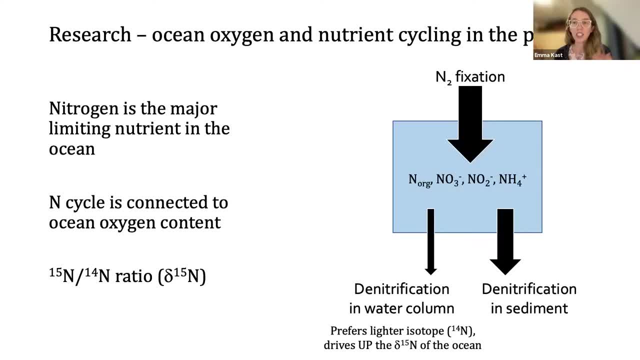 This can all be connected to ocean oxygen, because as you decrease the amount of oxygen in the ocean you tend to increase how much denitrification can happen And then you can change your nitrogen to change your nitrogen isotope values. So this kind of how we try to reconstruct the nitrogen cycle in the past. 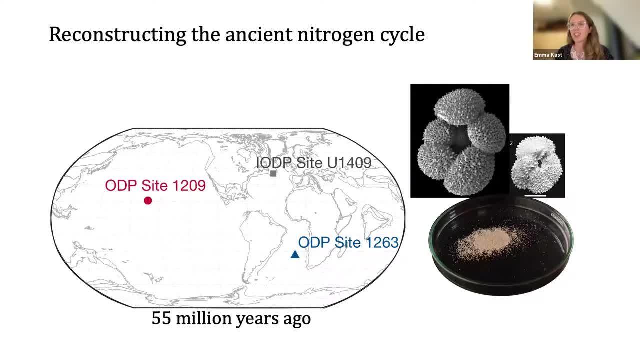 Okay, So again we turn to our trusty friends, the forma nephra, And in this case we're actually going to measure the nitrogen isotopes of tiny little bits of organic matter that are trapped within that carbonate shell. So that's like how we do these types of reconstructions. 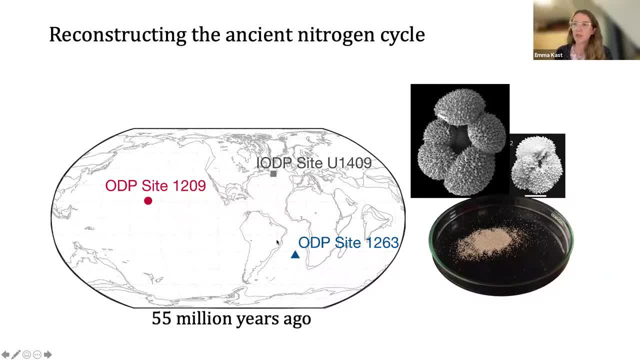 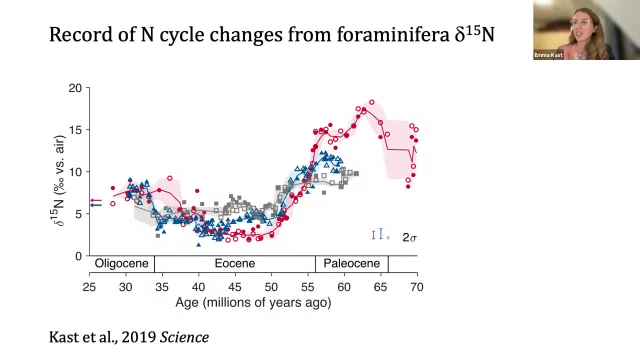 And in this case, for We're looking at sediments from three different sites around the ocean, And this is kind of the result of all this work. So I have to apologize here, because this age axis is the opposite way. And yes, just note that in your mind. 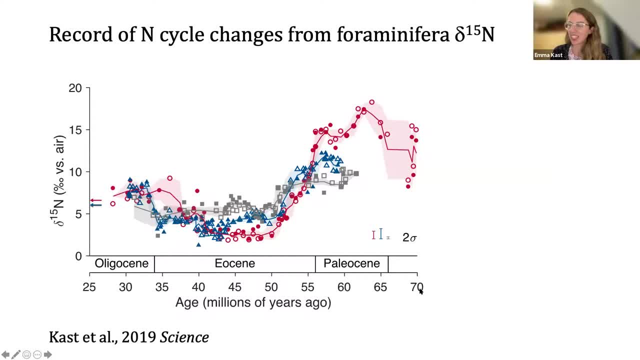 So this is actually the oldest side, at 70 million years ago, and we're going towards the modern, going to the left. Sorry that it's a bit confusing. And then on the y-axis, here we have the delta 15, so that nitrogen isotope ratio of 4 Amps. 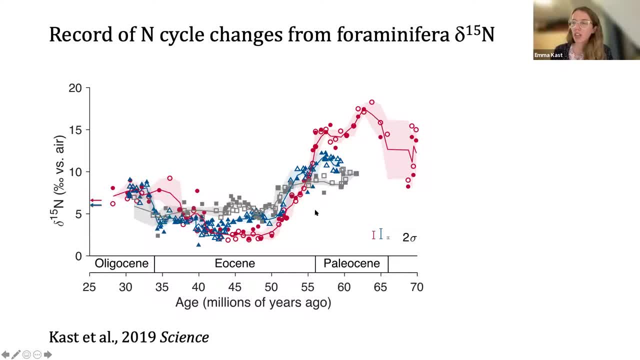 at these. the colors are just the three different sites. Okay, so just to kind of remind ourselves, we have this picture of the nitrogen cycle with these inputs and outputs, And really the key idea is that this denitrification in the water column. 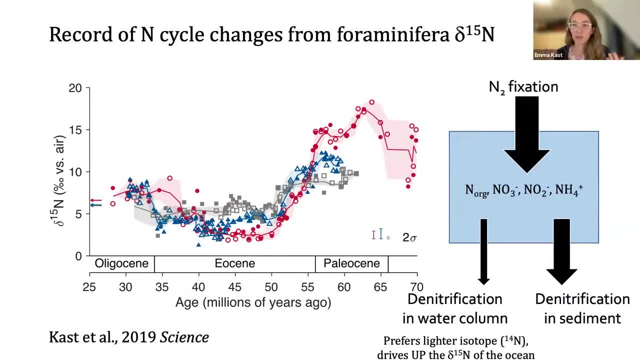 If it increases, then we're going to increase the delta 15 of nitrogen in the ocean, And if it decreases, we're going to decrease the delta 15 of nitrogen in the ocean. Okay, so let's use that frame to interpret this record. 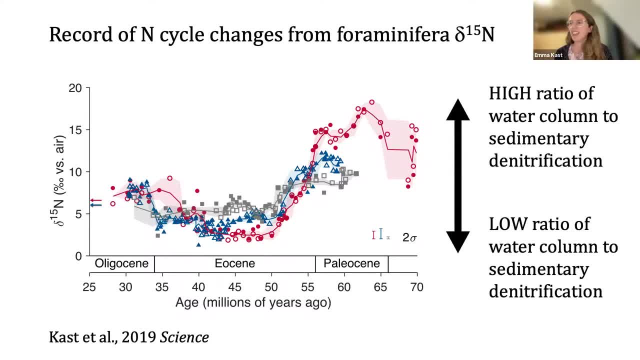 So, basically, the higher values mean higher water column denitrification, which also means less oxygen in the ocean, And the lower values mean lower water column denitrification. Okay, Okay, water column genotrification and higher oxygen. So if we look at this record, 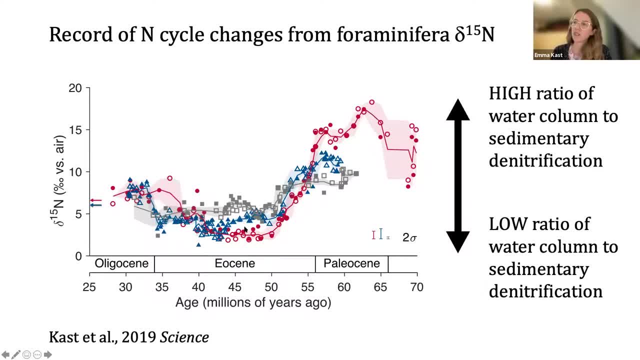 we have some really high values early on, and then they go, they decrease quite substantially into this kind of middle period, And so we can interpret that big change here as a decrease in the amount of water column genotrification, which also means that suboxia decreases. 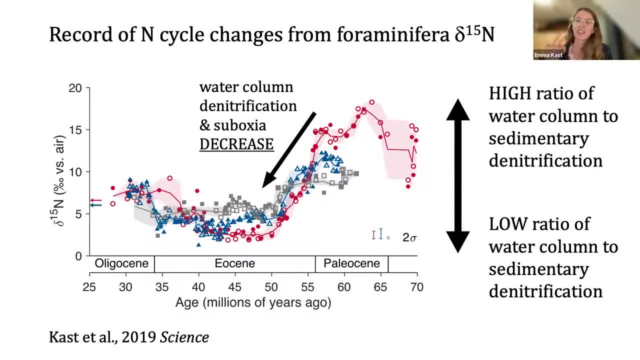 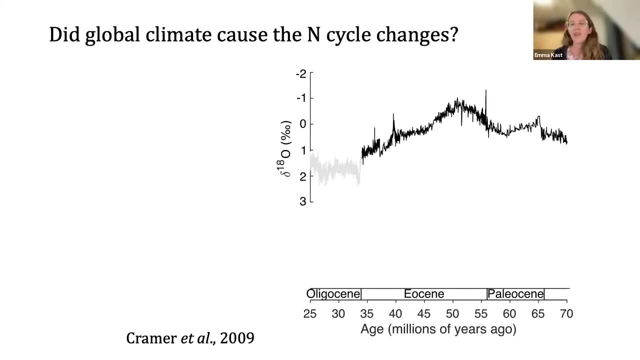 So we're lowering the oxygen, sorry, so we're increasing the amount of oxygen that's in the ocean over this time period. Okay, So, to tie this all back to this idea of paleoclimate, we're gonna compare how this kind of matches up. 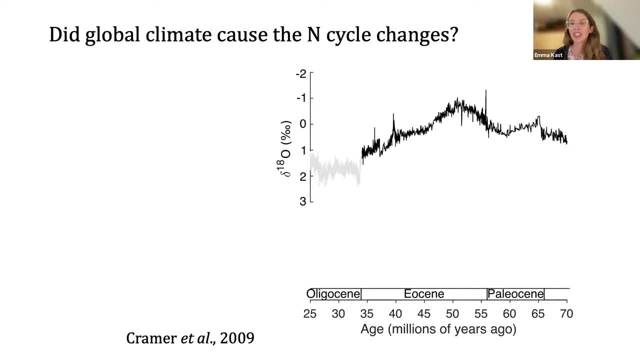 to the climate records, And we have a good reason to want to do this. The reason is that most of the time, we think of ocean oxygen as being controlled by the temperature of the water. This is a kind of straightforward solubility argument. 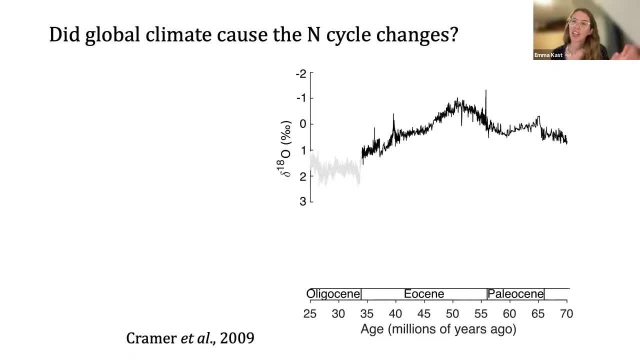 So if you have warmer temperatures, you tend to have less dissolved oxygen. If you have colder temperatures, you tend to have more dissolved oxygen. So when we, like, went into this project, we thought that we'd see some relationship to these global climate changes. 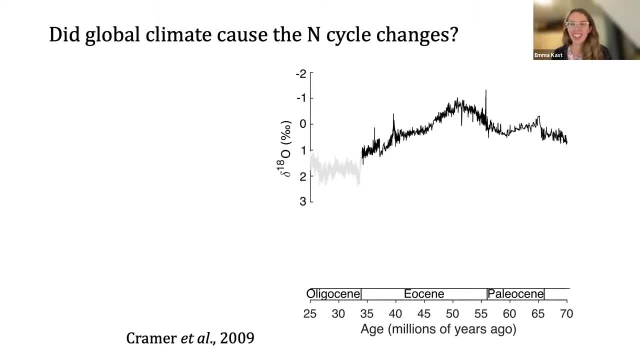 And so we're gonna explore that in this slide, and then I will be happy to take questions. Okay, So we have seen this before. This is our 4m oxygen isotope record, So this is telling us about temperature, And I'm plotting it again. 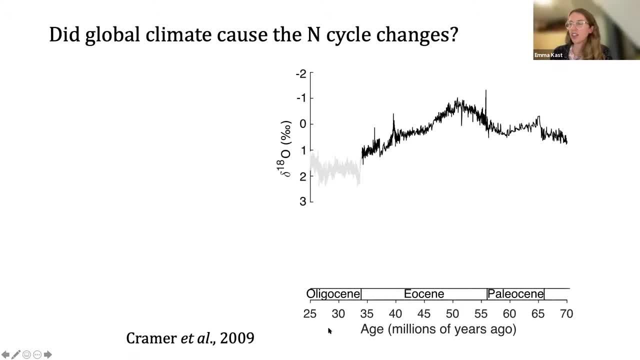 the oldest time period is here and we're going towards the modern, so millions of years ago. Okay, So with that solubility argument, higher temperatures are plotted upwards on this plot. So if we have higher temperatures, we're gonna have lower oxygen. 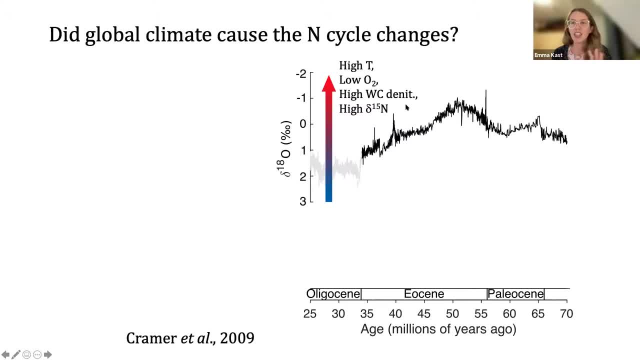 We're gonna have more of that denitrification that happens in the water, at the ocean, And so we should have a higher delta 15.. So is that what happens? The answer is basically no. that is not what we saw. 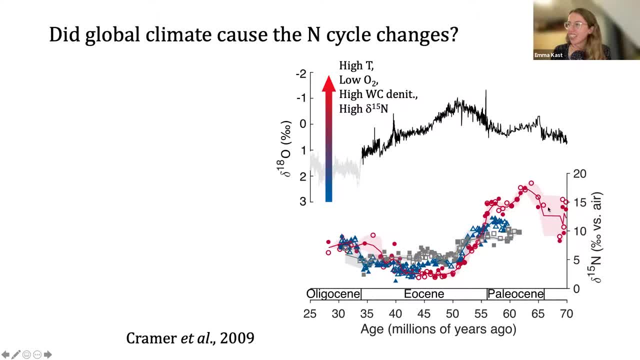 which was very surprising. So here again is this: nitrogen isotope records. This is, yeah, Telling us about what's going on in the ocean with the nitrogen cycle And to just highlight two intervals. So this interval, here you have warming and CO2.. 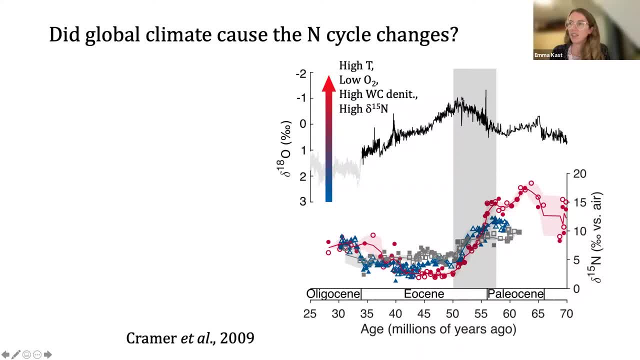 Okay, this increase in- yeah, increase- in temperature, But at the same time, we have this really dramatic decrease in the nitrogen isotopes, which is exactly opposite of what we'd expect. And then we also have this interval where there's cooling, but we actually have really stable nitrogen. 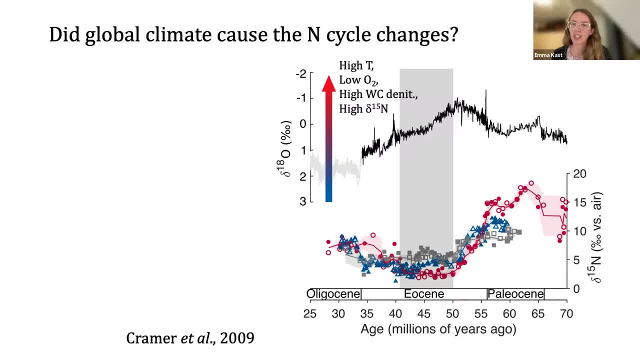 isotope values. So again, not what we were expecting based on this kind of oxygen solubility, temperature connection with the nitrogen cycle. So really, one of our conclusions from part like this research is that global climate was not the main driver of this nitrogen isotope record. 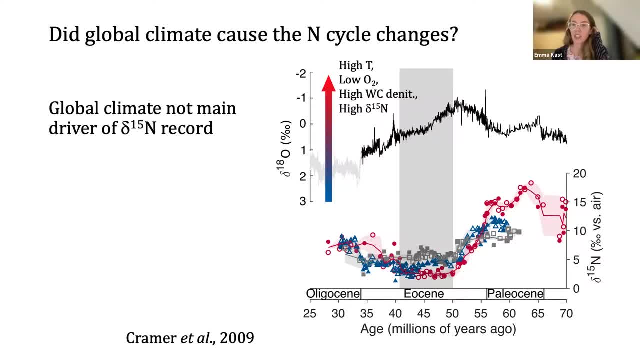 and was not driving these oxygen changes that we were seeing, based on the nitrogen isotope record. I'm not going to go into it at length, but our likely explanation for this kind of nitrogen cycle and ocean oxygen change has to do with the ocean circulation. So once you're looking at these kind of long timescales, 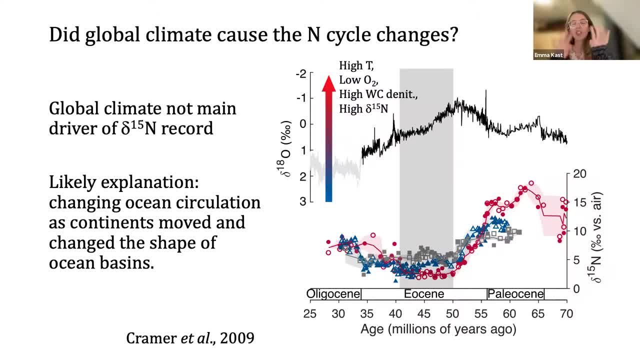 you also have to consider that the continents are actually shifting around and this changes the shape of ocean basins and that can change your ocean circulation, And so that's what we think is kind of our likely explanation for these nitrogen cycle changes in the Cenozoic. 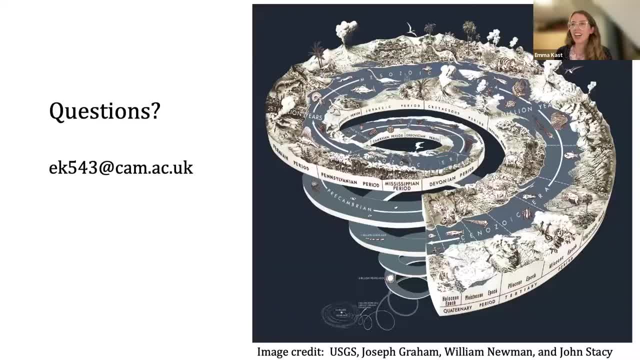 Okay, I know that was quite a lot and I'm happy to take questions. And if you also think of questions later, I put my email up there. Definitely, feel free to send me an email and I'll try to get back to you on reveals of all time. 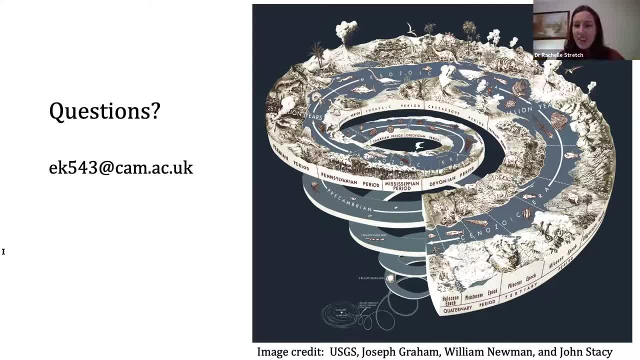 Thank you Brilliant. Thank you very much, Emma, for that overview. So do type in your your questions in the Q&A box. I see we do have one, but I was going to start off with a question: If you could just say something about how you obtain these for for Aminifera I mean. 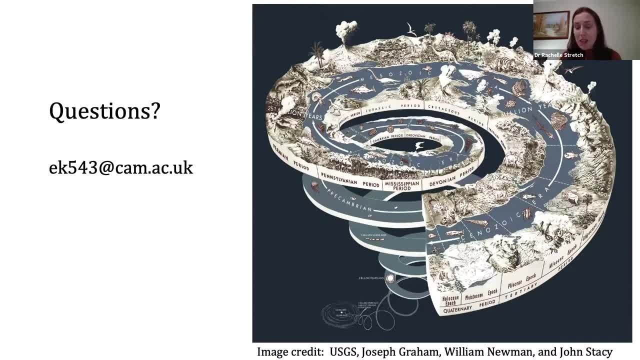 how do you go about kind of getting them And then getting the isotope information? Yeah, that is a that is a great question, Okay, Cause I, I, I, I love, I love how I get these. Okay, So there's, there's basically this international organization, consortia who do. 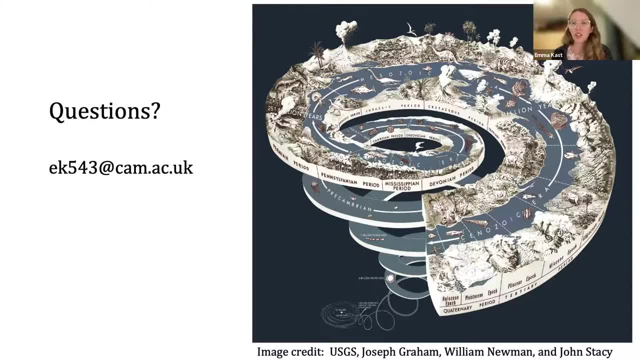 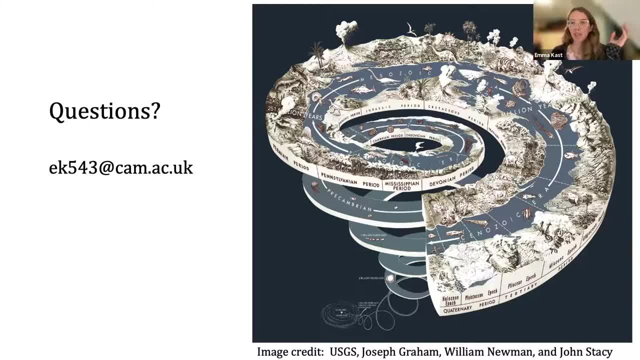 drill core, And so they kind of go around to different sites that have been, you know, proposed and vetted and et cetera, and they bring back drill core. So they're like circle, like tubes, They're about this big and they drill down in some cases. 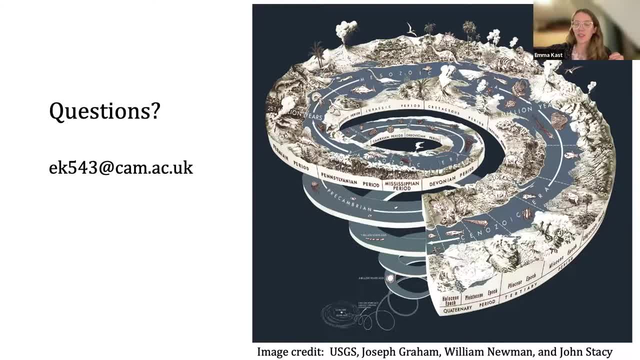 almost a kilometer or more into the bottom of the ocean and bring back these marine sediments that have forums in them and they also like other stuff too, then the super cool part is that, as a researcher, you can request samples um from this organization, and you know, they'll, they'll. 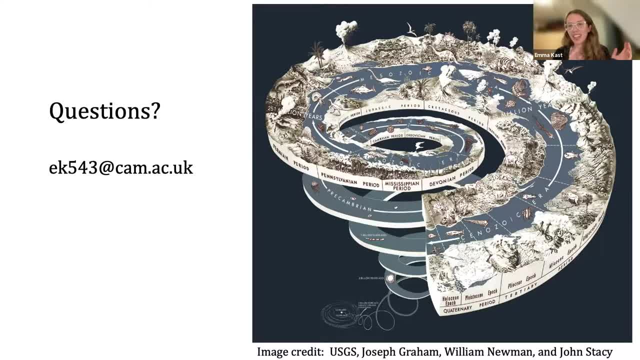 basically send you material. um, yeah, so that answers the like: how do you get the samples part? it's called- oh sorry, i should say the name. so the name is the international ocean. i think it's called discovery project now. so the iodp. yeah, that's great, thank you. so i'll go to a 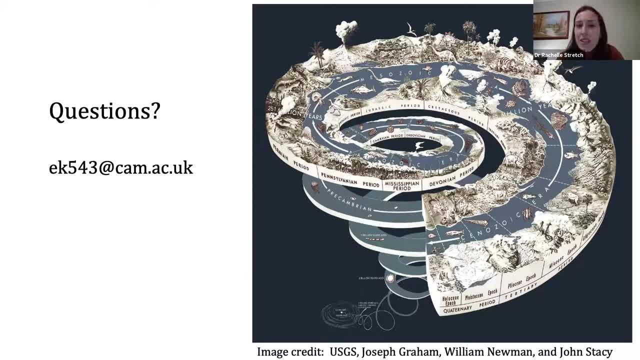 question that's in the chat: um, why did the antarctic get ice first? yeah, that's a good question. um, so one one reason is that the land mass of antarctica is actually much higher latitude than where the land mass is, and so i think that's a good question. um, so, i think that's a good question. 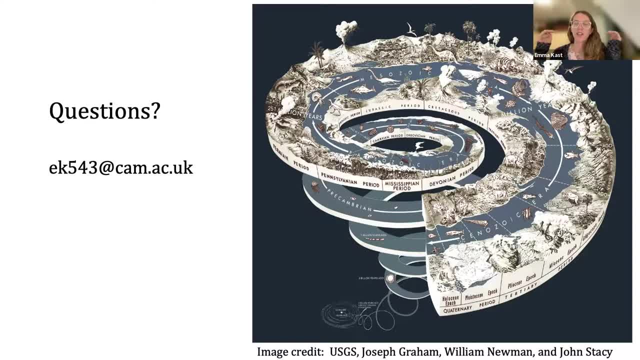 where we have land in the northern hemisphere. so we don't right now we don't have any land in the northern hemisphere. that's actually on the poles. so in general antarctica is like farther poleward um than in the northern hemisphere. there's also this like interesting oceanographic: 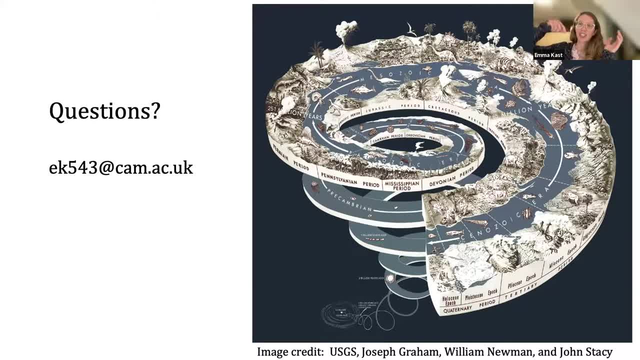 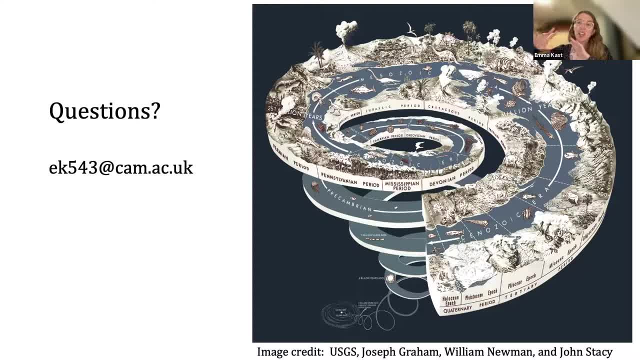 described to me is it basically kind of isolates antarctica, um, so it's harder to like get warm air to antarctica, so it's kind of like separated away from everywhere else because of, yeah, all these kind of dynamics. yeah, that's great, thank you, and sort of thinking about your, your own research, as 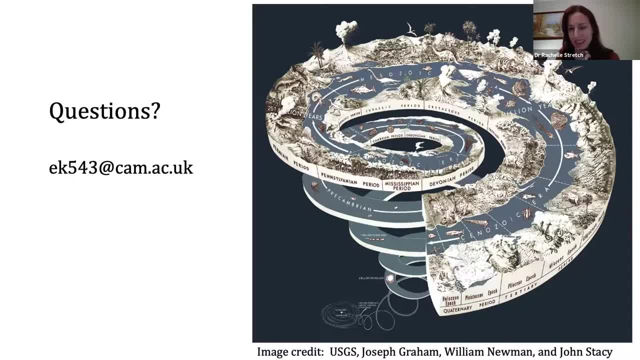 well, you obviously have this hypothesis and then it wasn't as you expected. uh, i mean, how did that kind of feel then, when it was not the results that you were thinking of and and is there any way? you've obviously come up with an explanation, but is there any kind of further research now that you can, you can be doing to? 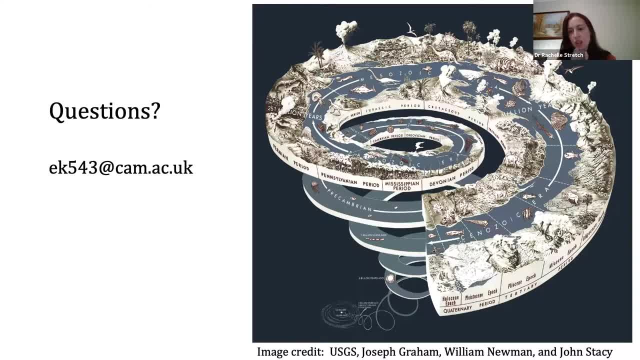 kind of test, that explanation that it was about the kind of the continents moving and changing in basins, yeah, as to like how it felt it. honestly, it's like i guess there was like the initial like what, like what is happening, but on the other hand i think it's it, um, it's exciting because you, yeah, it's something to 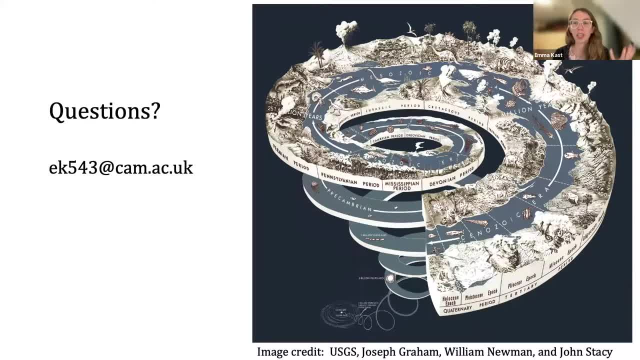 figure out, and it means that we don't have a, we didn't have a complete picture of, um, these kind of nutrient oxygen temperature dynamics, and so it's quite interesting to try to like figure that out and to be part of figuring that out, um, in terms of yeah, is there anything else to do? it's. 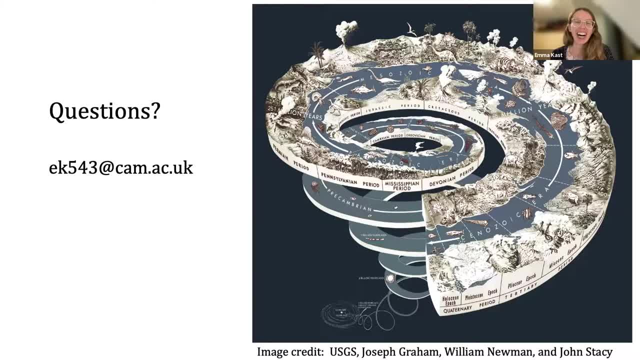 of course, yes, there is always one um, oh yes, i could go on and on, so, um, yeah, let's say so. one thing um that i'm actually working on here as well is this time period where we saw that nitrogen isotope change. um, it's this really. 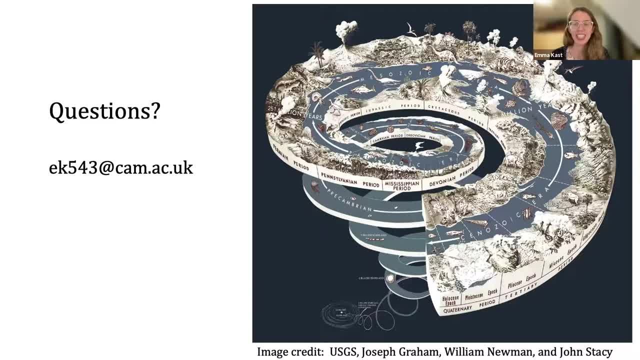 dynamic time. there's a. there's a lot going on in other geochemical cycles as well, but we're not quite sure how they all relate to each other. so, as an example, um, and one of the things i'm studying here is at a similar time, the sulfur cycle, which is it's connected to, kind of it's also connected. 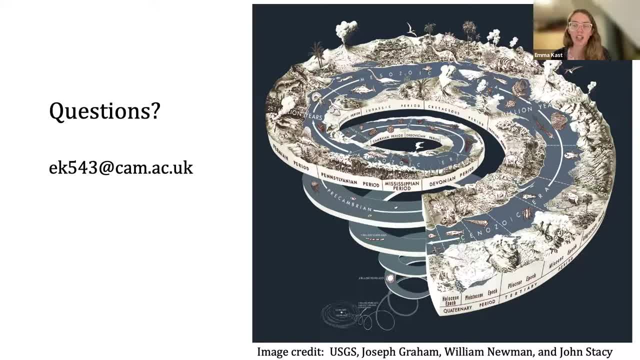 to ocean oxygen and the carbon cycle, the like biological cycle. um, it also undergoes this like profound change at a similar time, but we're not sure if it's at the same time and we're not sure exactly how they're connected. so, um, that's one of the things i'm working on here- is, like, how does the nitrogen? 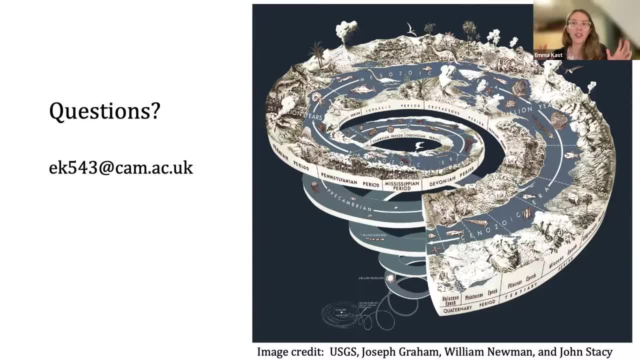 cycle really connect to kind of the other ocean biogeochemistry, that's that's happening at the same time and why did those things happen? and yeah, excellent. so another question in the chat and do feel free to to type any more in there. so question about the denitrification um is. 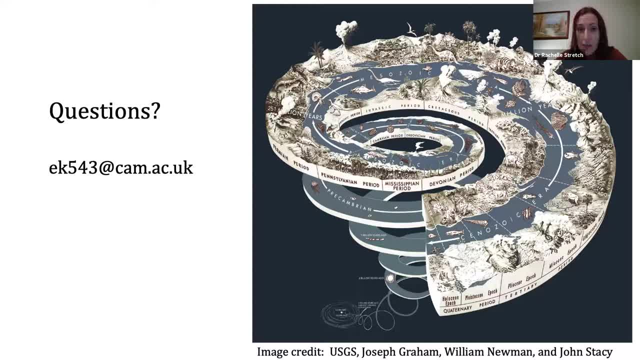 denitrification happening now, as it did in geological time? and can you check theories of ocean chemistry by studying contemporary ocean chemistry? And can you check theories of ocean chemistry by studying contemporary ocean chemistry? contemporary ocean chemistry: Yes, absolutely. I would say it's almost a requirement to understand. 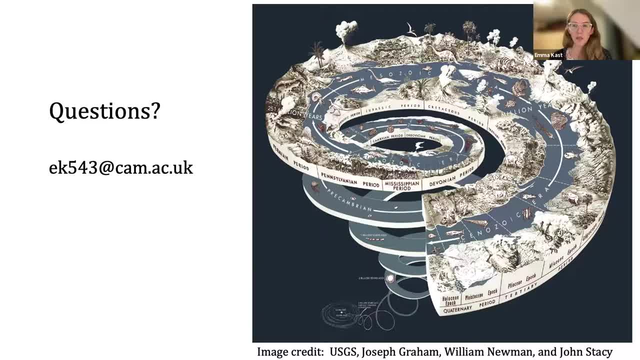 the modern ocean chemistry before we can really properly study the past, in the sense that a lot of the way that we think about the nitrogen cycle is based on our understanding of the modern nitrogen cycle. So, for example, I put up that little box diagram with the ins and the outs. 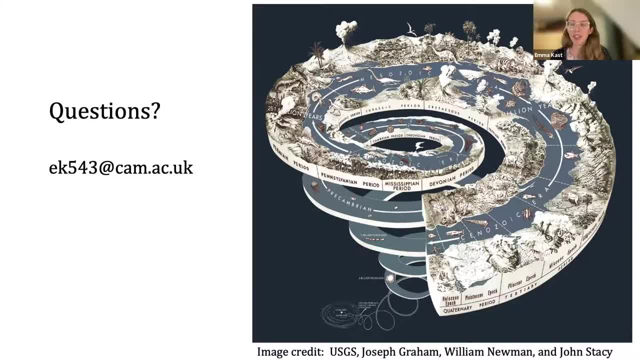 We know that that's how it is because people have gone into the modern ocean and taken a bunch of measurements and tried to figure out what's happening to nitrogen in the modern ocean, And so we can kind of take that framework and try to see how that might have changed in the past. 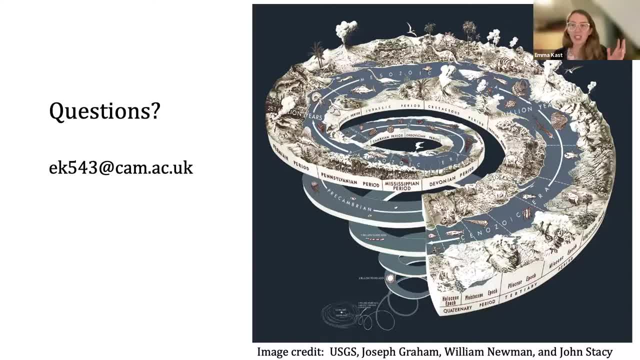 So yes, absolutely, Like we try to like talk back and forth to each other between the modern and the kind of paleo side of things, Yeah, absolutely, And I didn't know whether to pick you up when you said there was the longer answer. 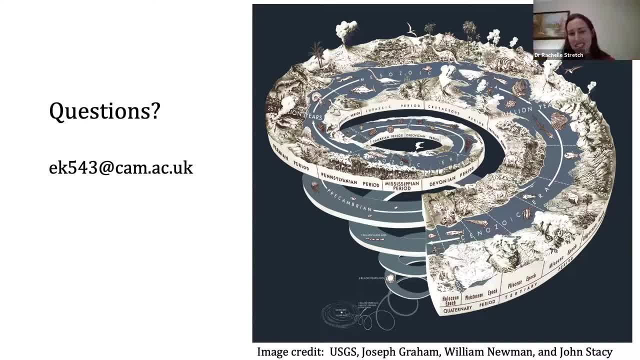 The white climate has changed over the center zone and the kind of the changes in CO2 as well, So I didn't know if you wanted the opportunity to say a little bit more about that. Yeah, I could, I could say a little more. It's definitely a more involved answer. 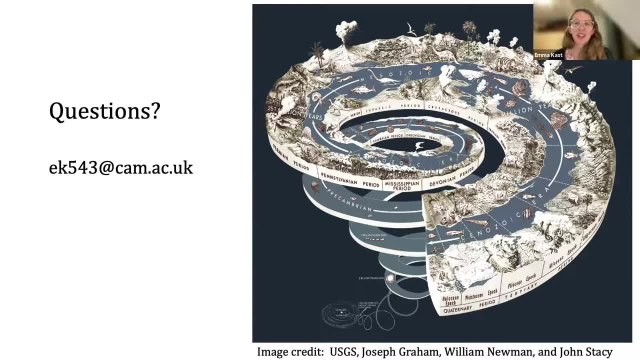 But it's also really cool. So on these long timescales, to our best understanding, the thing that controls atmospheric CO2 is this interesting balance between basically CO2 going out of the atmosphere And the stuff that's going in is coming from volcanoes, basically. 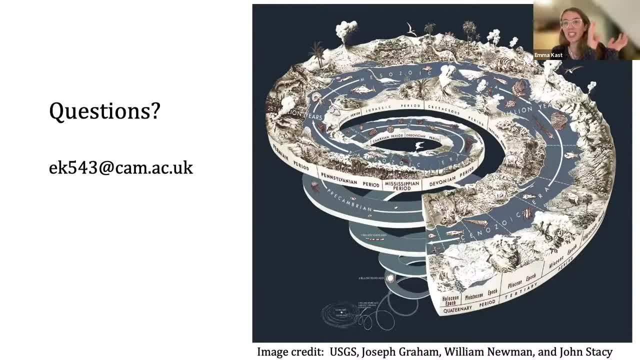 Right. When a volcano erupts, it emits some CO2 and that ends up in the atmosphere. If that was all that was happening, then over time we'd just steadily accumulate CO2.. It would just go higher and higher and higher. 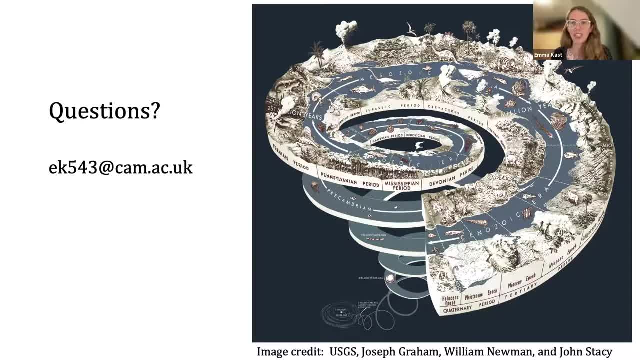 So to balance that out, in the Earth system what happens is CO2 in the atmosphere actually reacts, basically with rocks, So a particular kind of rock is called silicates. So the CO2 plus these silicate rocks, they like, react together and basically extract the CO2 from the atmosphere. 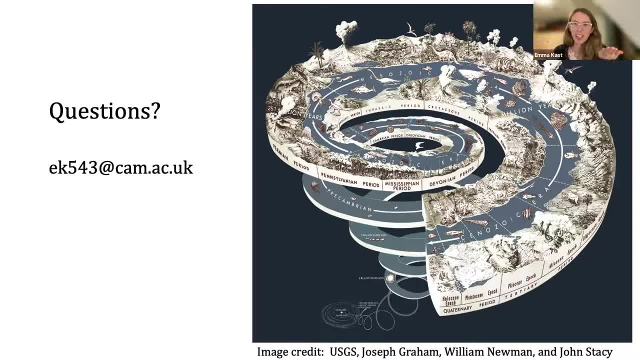 And when these things are in balance, then the CO2 in the atmosphere stays the same. And so for this, like Cenozoic climate change and the CO2 changes, yeah, one of those things has to have been affected somehow, like for some other reason. So one hypothesis- and this is definitely gets into like more of a debate than like for like full understanding- But one of the hypotheses is that during the Cenozoic you have the buildup of some really large mountain ranges. So mostly people talk about the Himalayas And when you build mountain ranges you like expose a lot of like fresh, like tasty rock And it basically makes that output like it sucks down more CO2 than is being put out by the volcanoes. 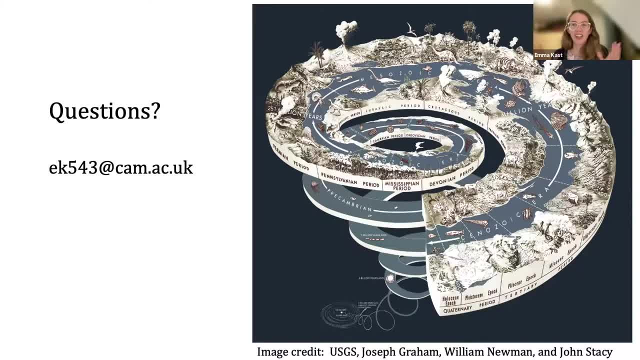 And you start to draw down some of the CO2.. So that's yeah, that's one of the main hypotheses. Brilliant, That's great. I wanted to get volcanoes mentioned in that, bringing my own past, Thank you. Are there any more questions out there? 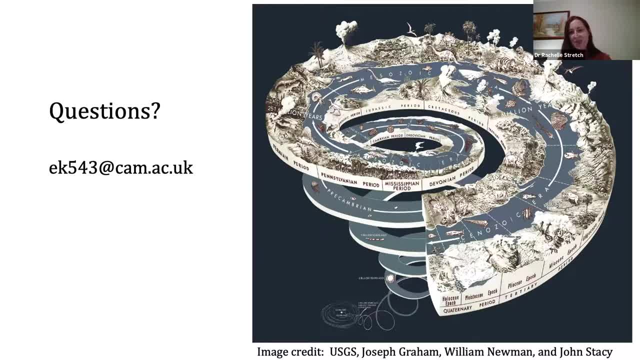 Do feel free to type them in the chat, But if not, we'll. I think we will sum up there. It's a huge task. Yeah, It's a huge task. Yeah, I think it's going to take five minutes. 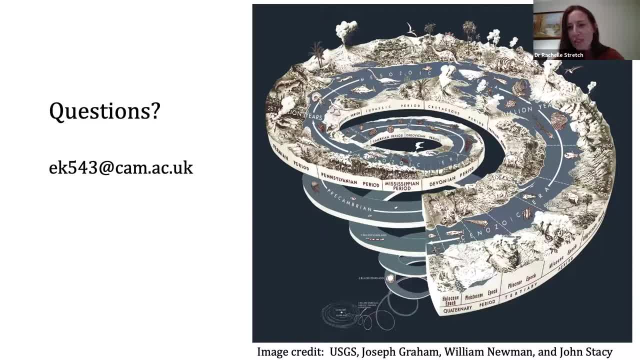 huge thank you to Emma for an overview of the climate over 65 million years. obviously, we're we're very focused on the present day at the moment but, as you say, having that understanding over such a long geological time period is so helpful to understanding and indeed, modeling. 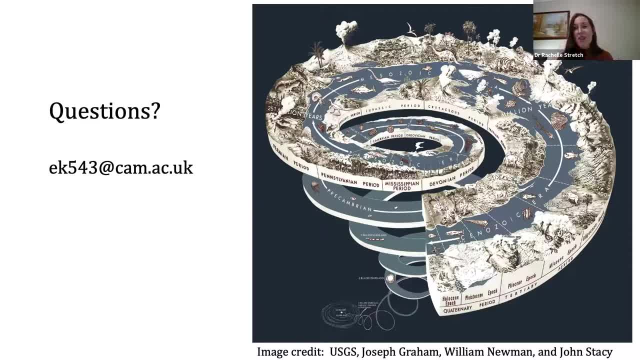 the present day. so thank you so much for that. we do have more events coming up in our climate change series. we have sort of entrepreneurs involved in climate change. on the first of November, a business panel and how you balance both profit and sustainability. on the 9th of 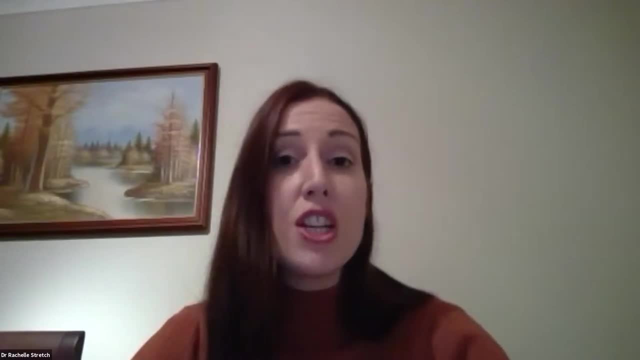 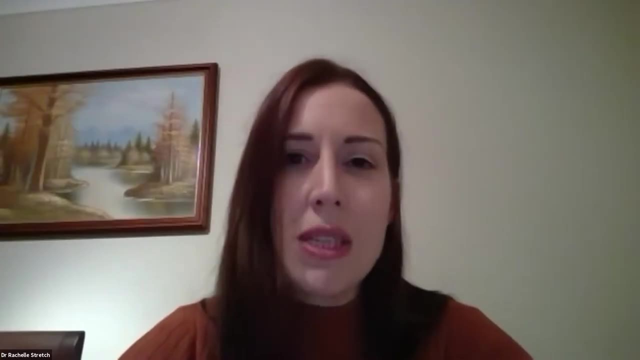 November and another one of our fellows talking about climate change and climate justice in Africa on the 10th of November. so do join us, for those signups are all via our website, but we will be recording them and you'll be able to watch them through the Trinity Hall YouTube channel as well. 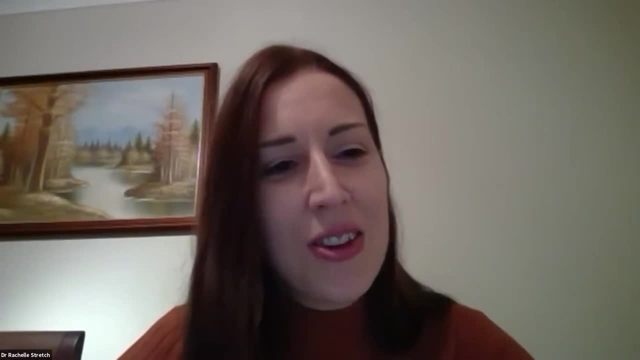 so thank you to you all for watching, and a huge thank you again to Emma, and hopefully see you all soon. thank you, bye you. 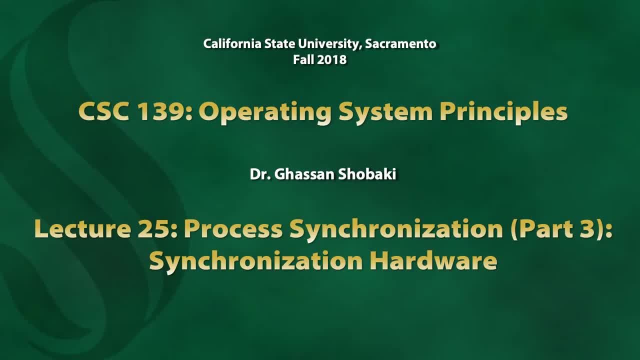 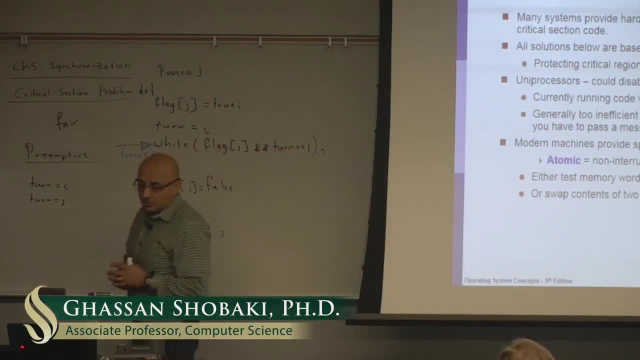 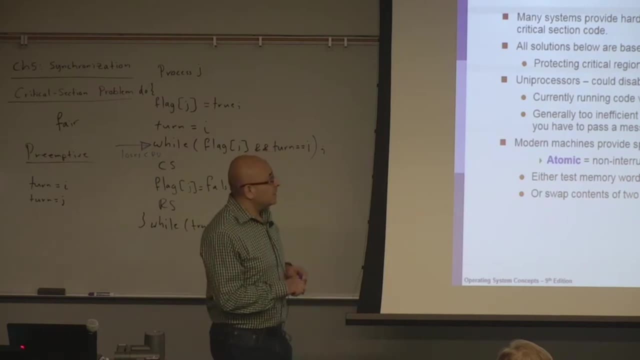 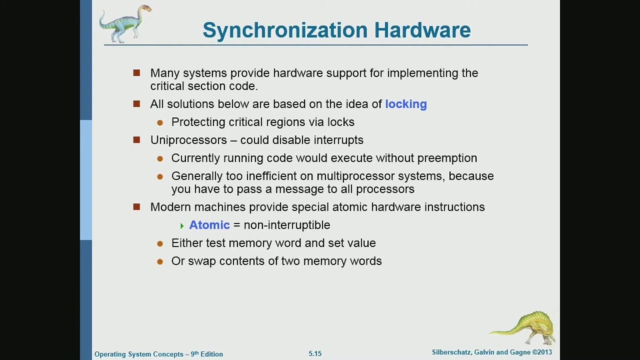 Now we talk about synchronization hardware, about hardware instructions for synchronization. Before we talk about this, we just indicate that on a uniprocessor system it is possible to solve a critical section problem by disabling interrupts. Remember that if a process is guaranteed, not